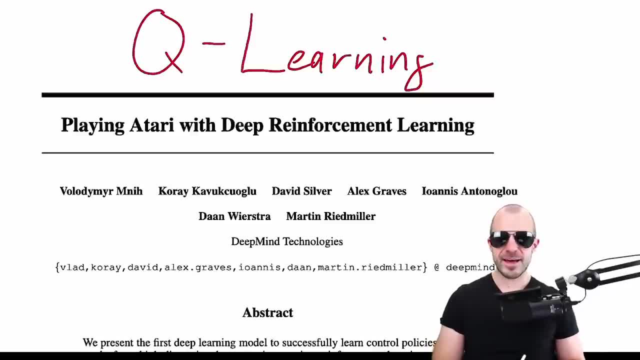 but everyone's speculating around what that could be And I thought it'd be good to go back to the basics and look at what is Q-learning and what does it do, and how has it been used recently or not so recently, namely in this paper right here, Playing Atari with Deep Reinforcement Learning by. 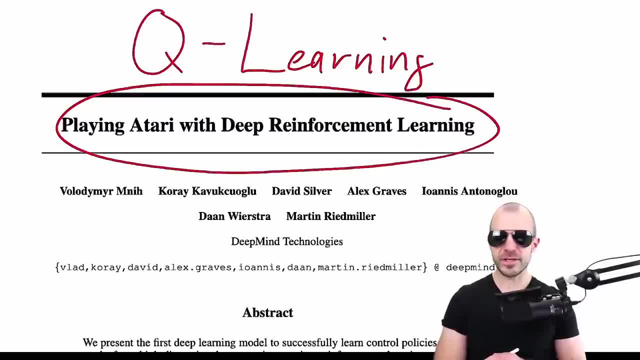 DeepMind, which was one of the first papers that really catapulted DeepMind to the forefront of everyone's attention. So it's not going to be sort of state-of-the-art research today. it's more going to be a basic introduction into Q. 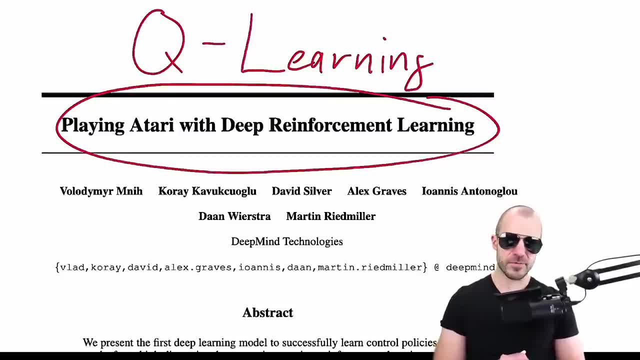 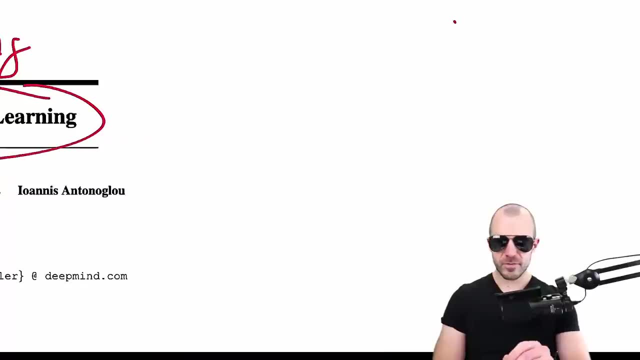 Q-learning. I've actually done a video on this particular paper before. If you want to know more about this paper today it's really going to be about Q-learning in general, So let's dive in Q-learning. we're in the field of so-called reinforcement learning And again we'll keep 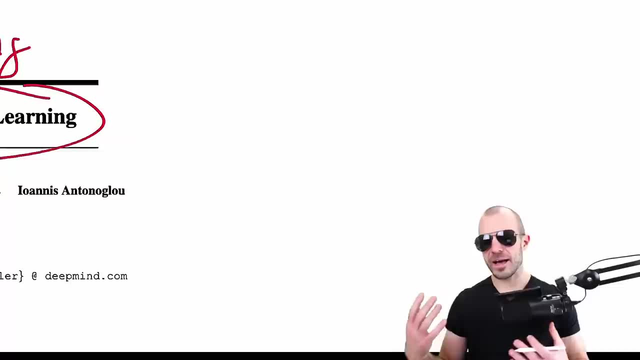 an eye on the application, how that might apply to a language model or something like this as we go through this. But in the basic sense, in reinforcement learning, you have your agent over here. that is the ugliest A I have ever seen, So you'll have your agent. 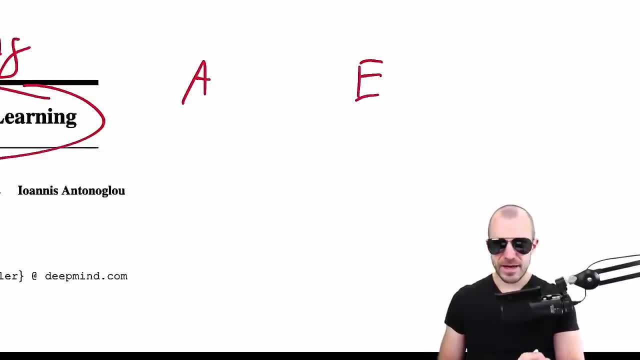 over here and you'll have an environment And the environment is giving the agent what's called an observation. O, Okay, the agent is going to react to that observation and then reply with an action. A, The environment is going to take that observation and it's going to react to that. 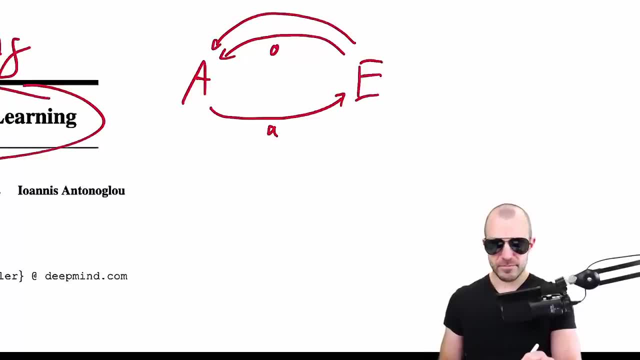 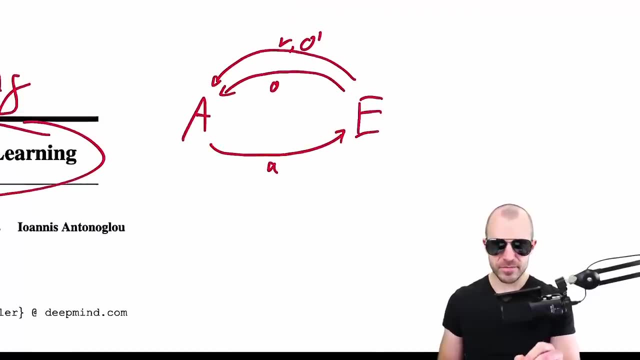 action and give the agent a reward. and a next observation. Okay, and this is the basic cycle in reinforcement learning. This is the most basic concept. the agent gets these observations from the environment, then responds with actions based on those observations And the environment. 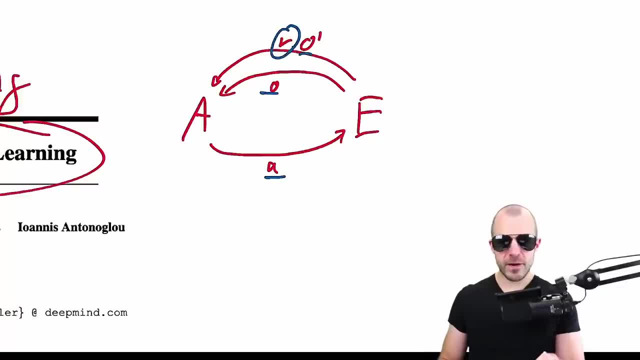 after the first step, it always gives a reward how good the last action was. Now there are multiple configurations, And there are multiple configurations and there are multiple variations of this. So the one simplification we're going to do today, let's say, is that we're 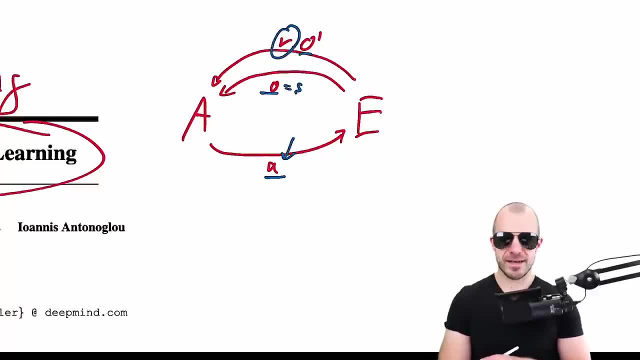 going to say the observation is always equal to the state. This is so called Markovian, fully, fully observable decision process, And that's just going to simplify things a lot. So when we say observation or when we say state, today will mean the same thing. Think of a chessboard. 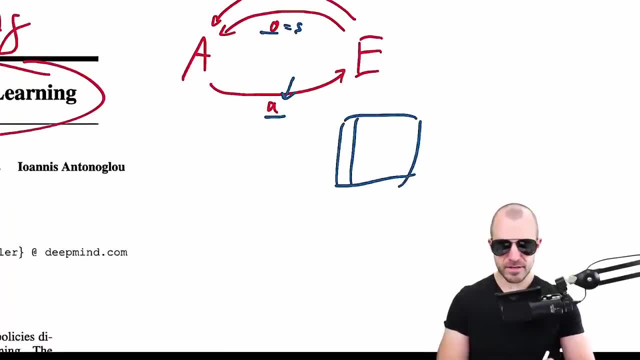 You observe the chessboard, as it is okay, here is maybe a simplified chessboard. you observe that you know the, the rook is here and the queen is here, and so on. You observe it once And that's. 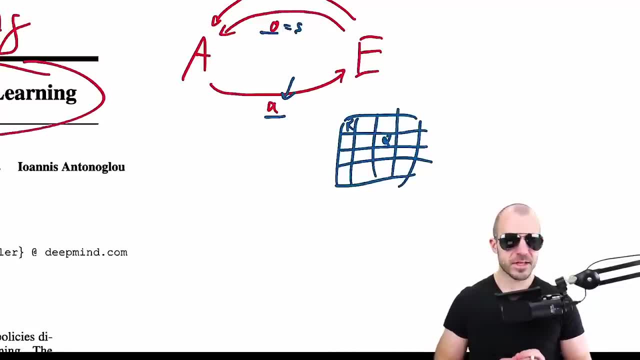 everything you need to know. That's the whole state of the game. There's nothing hidden. there's nothing dependent on something in the past which is actually not true. in chess, whether you can castle or not is actually dependent on kind of the past history And 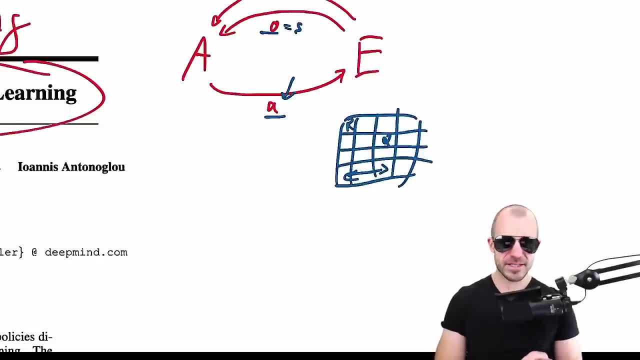 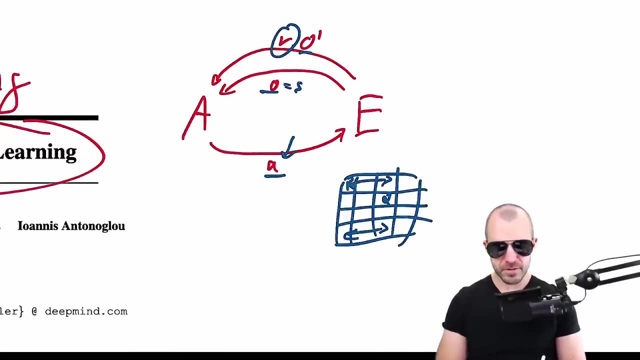 today, we'll also just ignore that. So you're in a given state and you're asked to make an action And that will lead to some reward. Now, in chess you already see that that's not really true in the colloquial sense. So if I move the rook over here, maybe that was a really bad move. Maybe that was. 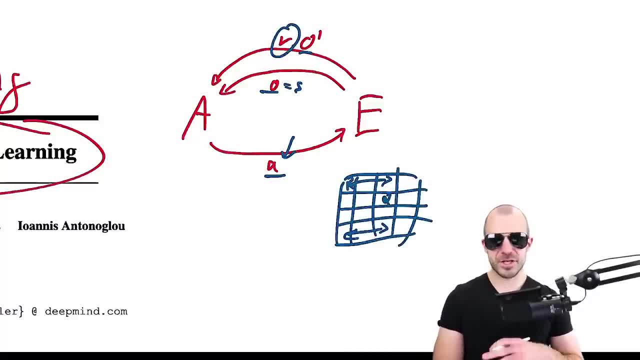 a really good move. It doesn't matter unless it's a checkmate. I don't get any reward at all, right? So my reward from the environment in chess is whether I have won or lost the game, And that only happens at the very end of the game, No matter. 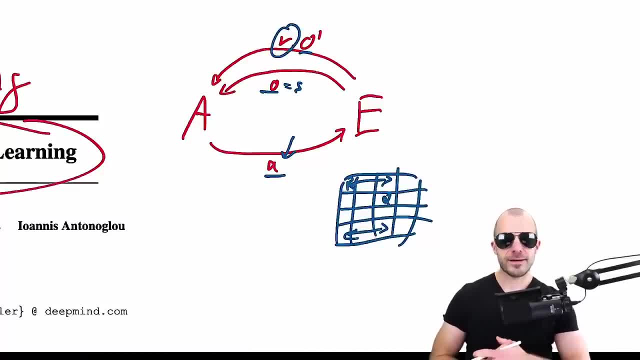 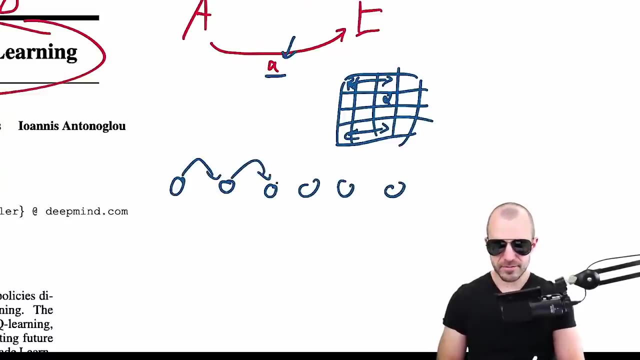 how good my moves are in between. I will not get any reward from the environment until the very last step, And that's a problem in reinforcement learning. So I can go from state to state, from step to step, I can go through this game and all, and I only get a reward here at the 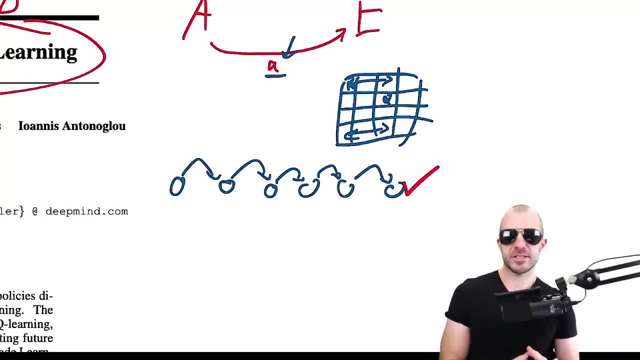 very end. Now, this is a very tricky situation for a system to learn, because how are you going to know whether the move you made here was ultimately the correct move? you have a very similar. you have a very similar challenge when you do like sequence to sequence learning with. 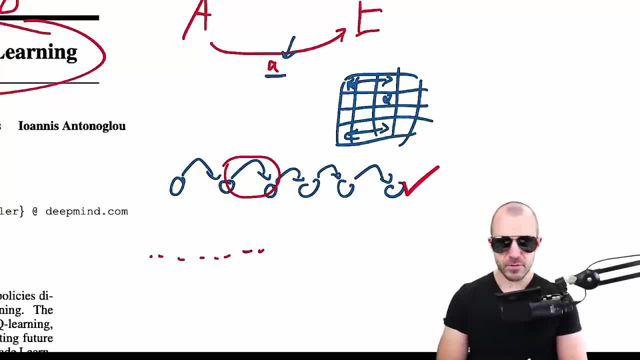 language models, because first you go through a sequence right and then you output the sequence over here. So this would be the encoded stage And then from here on, you'll decode And as if it's, as if you wouldn't get a loss, each token that 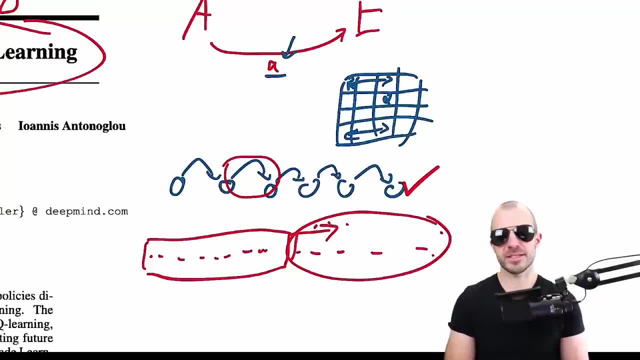 you produce, but only at the very end. someone would look at the whole sentence and say, well, that's pretty good or no, that's pretty bad right. And in fact that you know that's what we do when we do reinforcement learning, even for RL. 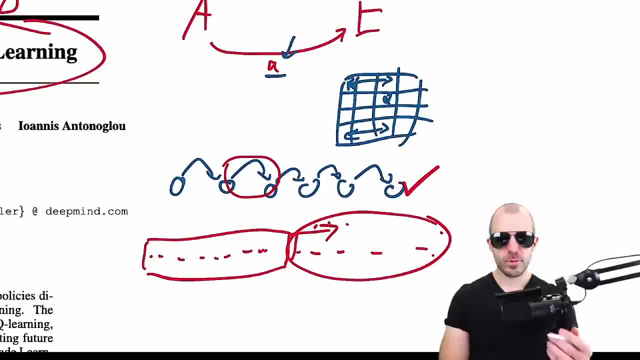 So reinforcement learning doesn't necessarily mean you only get reward at the end, But many environments are structured such that only after you've sort of completed the entire episode you get a reward at the end And you need to sort of figure out what was good and what was bad. that 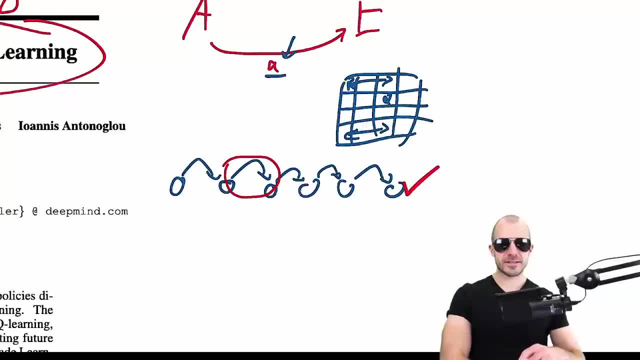 you've done in the meantime, And Q learning is one way that you know is kind of good at, let's say, mitigating that and doing this credit assignment. So the assignment of you know this actually depended on oopsie. 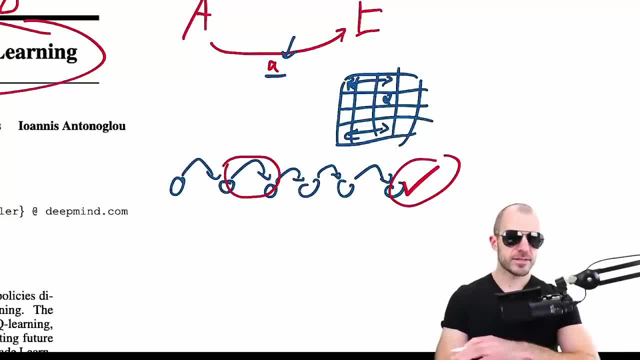 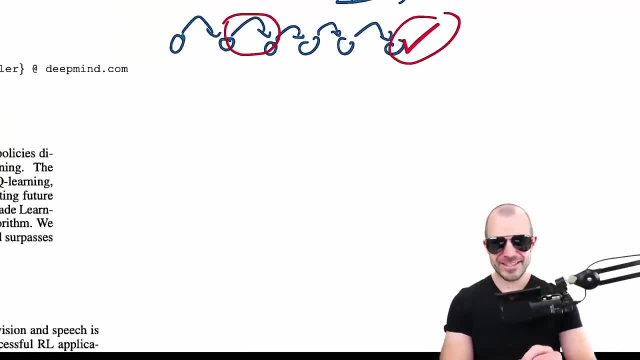 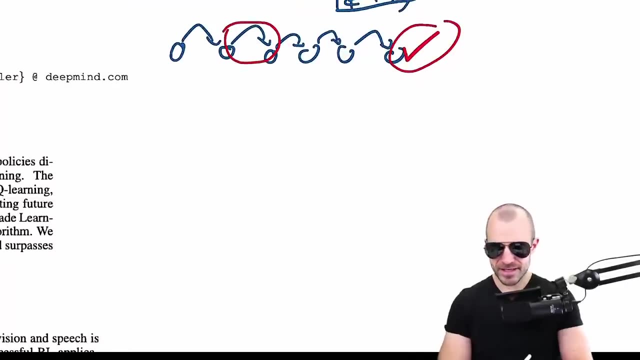 depended on moves that I've done before. So how do we go about this Formally? well, let's not go too formal. we have this is called a Markov decision process, fully observable, as we said, and that means that I'm always in some kind of a state. I take an action, I go to a next state. So 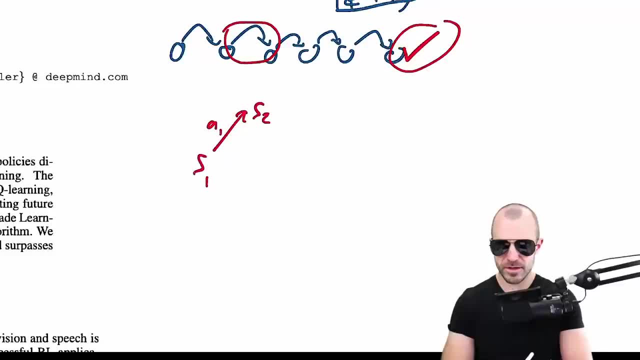 state one, I transition to state two by doing action one. If I did action two, instead I'm going to transition to state three, Maybe from state three. if I do action one, I transition to state two and so on, So I can move. 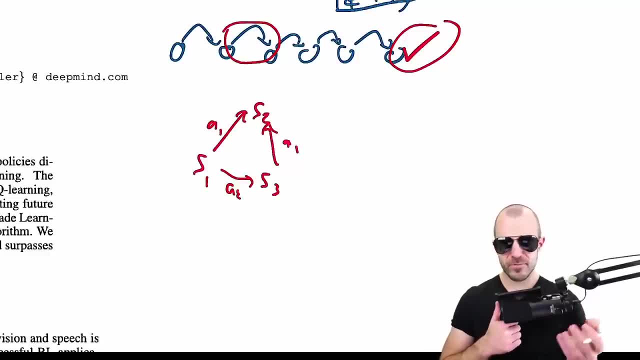 around these states by performing these actions. Also, we're just going to consider that you always have the same actions available in no matter what state you're in. It's also not entirely true, But so I need to figure out. I'm in a given state, right, And I need to figure out what action. 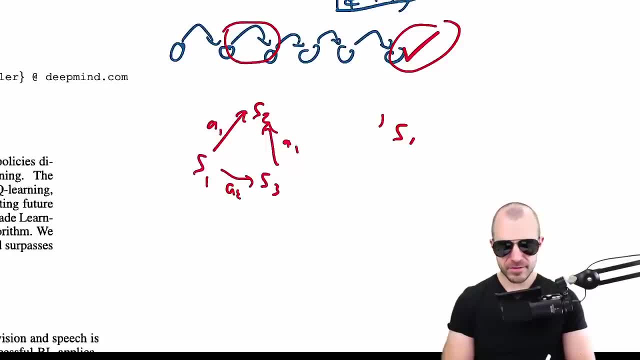 should I do? And one way to go about that is to have a function that takes in a state and gives me an action. That is that that is possible. That is, if you do any sort of actor, critic, reinforcement, learning or something like this. 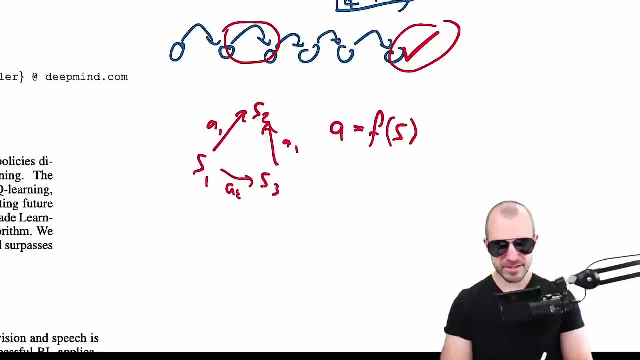 policy gradient methods. they do this, So they train a, they learn a function, that you input, a state and it's going to give you an action And it doesn't explain how or why or anything like this. Today we're not going to do that. we're going to do something different When I say I'm going to 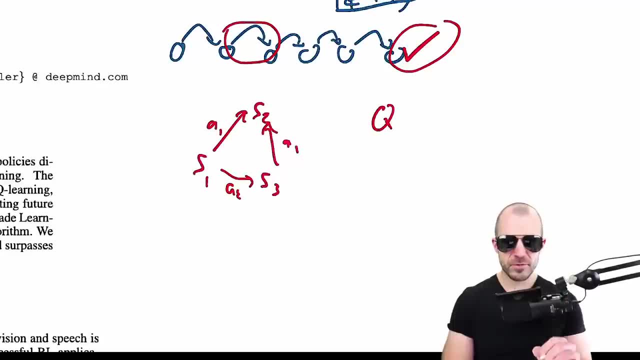 define a function, q, And what q is going to do. q is going to take in a state and in a proposed action, a proposed action. So you're in state s And you're saying, if I did task a, what would my total reward? 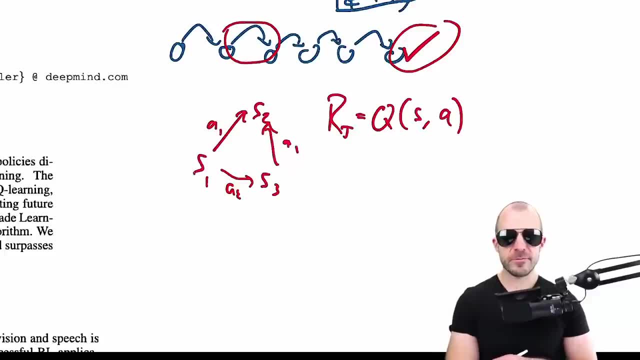 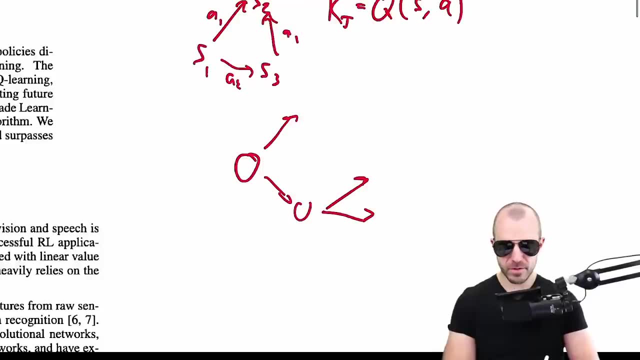 reward b if I did action a, so you're in some state here, right, you could go here. you could go here. from here you could go in many different places And at some point that there will be end states. 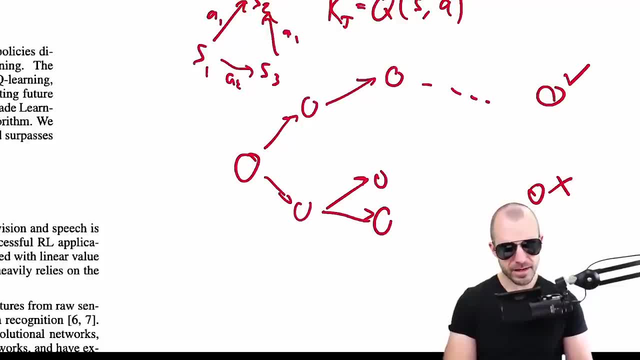 And in the end states: this is a good one And this here might be a bad one, And you don't know how you, how you get to to these right. So you're in state, in this state here, And you're asking: 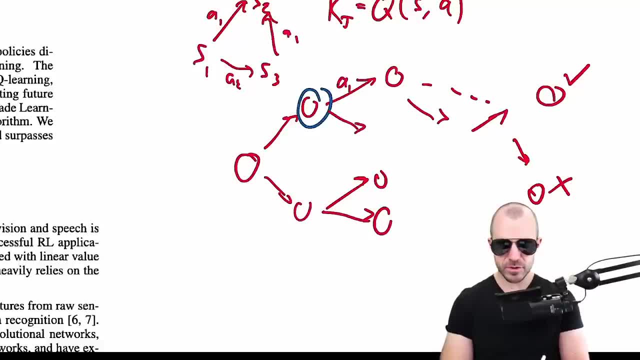 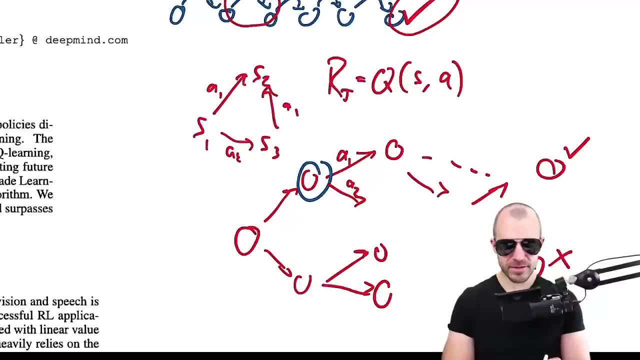 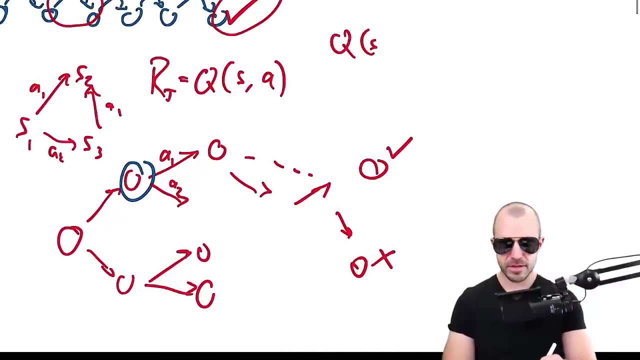 yourself: which action should I do? Should I do Action one Or should I do action two? Well, if you had this function, what it would tell you is: okay, if I plug in, if I plug in a one here, let's say I plug it in, I'm in state s, this is state s. 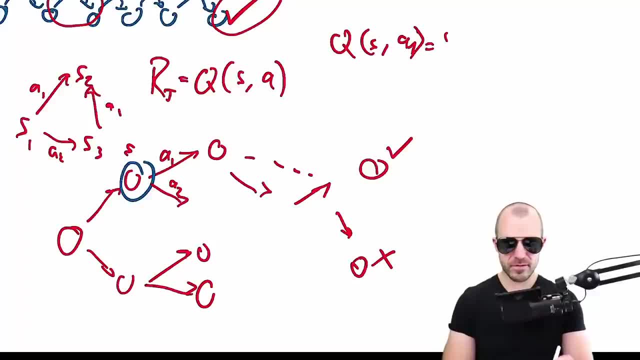 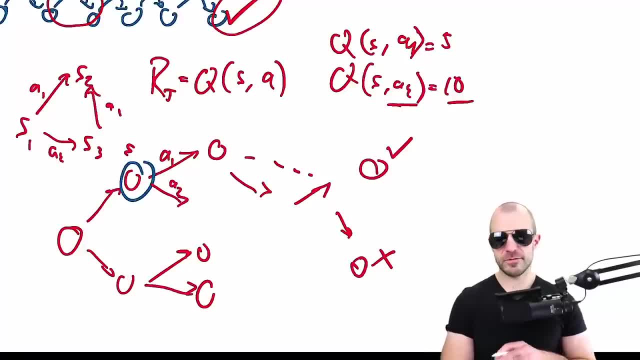 So I'm going to choose a two. So I'm going to choose a two. So the Q function is a function. let don't worry how it comes about. the Q function is a function that in current state you give it a proposed action, it tells you how your total reward from here on out, how much that's going to. 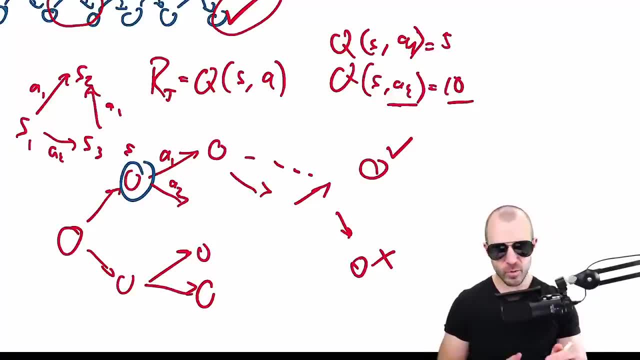 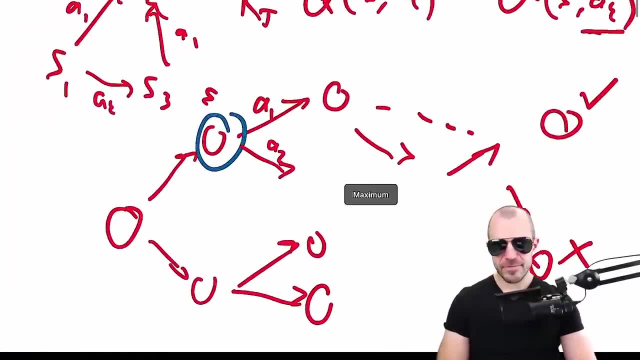 be if you now do action, whatever action you plug in. that is missing a little bit of information. if you've realized that, And namely, even if I do action a two here, I'm going to be in this state, I'm still going to have 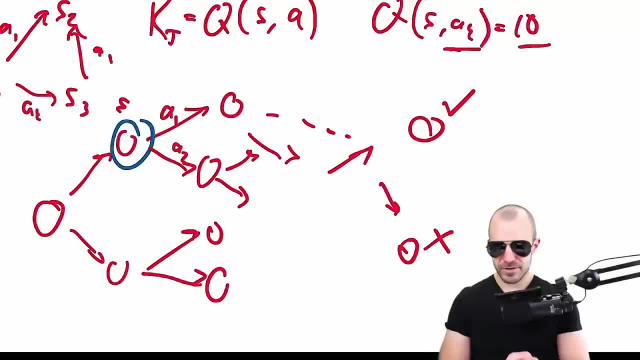 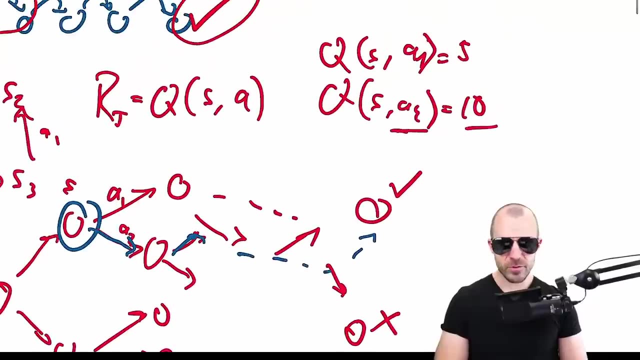 options even after that right. So just because I now decide to do a two after that, I can still, and probably will, have to choose many more times what to do until I finally reach some sort of good or bad end state. So in order for this Q function to be well defined, I also have to specify what I 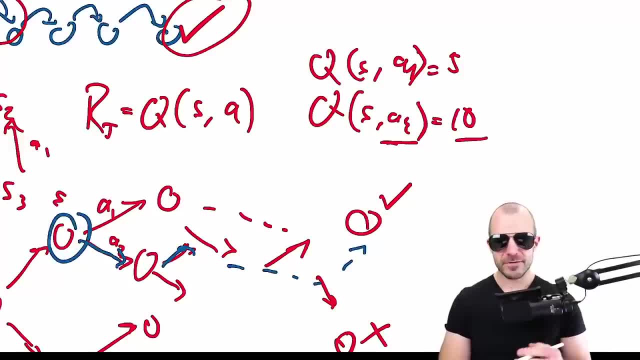 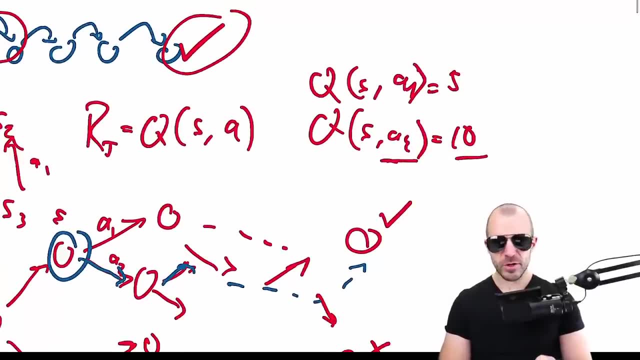 do So. in order for this Q function to be well defined, I also have to specify what I do after that. And what I do after that is that's called a policy. So a policy, and I previously called it F. but 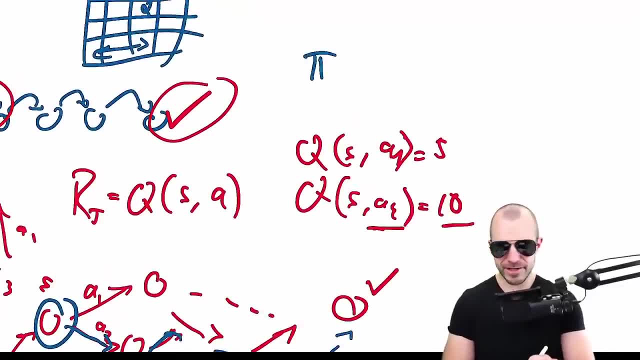 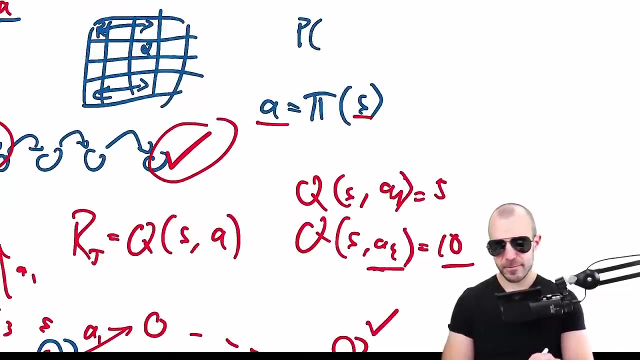 technically or not technically. commonly it's called pi, So pi of s. This is a policy. you give in a state s and it tells you do action a. Sometimes this can be formulated in a probabilistic manner, So you can say: my probability of doing action. a given state s can be defined as this, So: 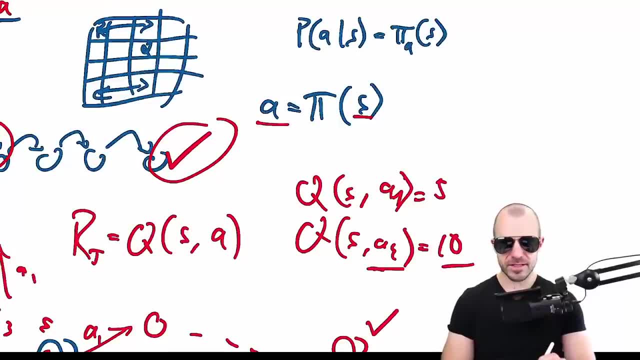 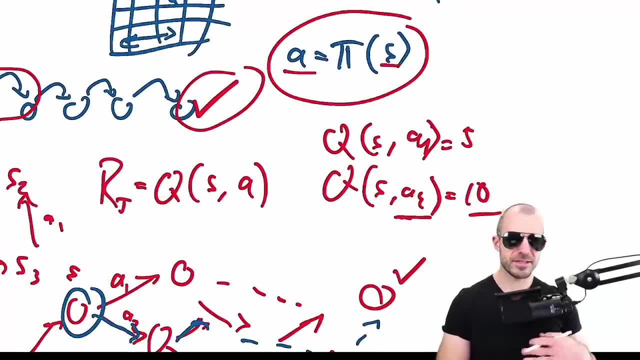 it's going to give you like a probability for action, a given state s. But we can also go the deterministic case right here and say a policy, you give it a state and it's going to tell you: go left, go right, go up, go down. Note: the policy says nothing about reward. 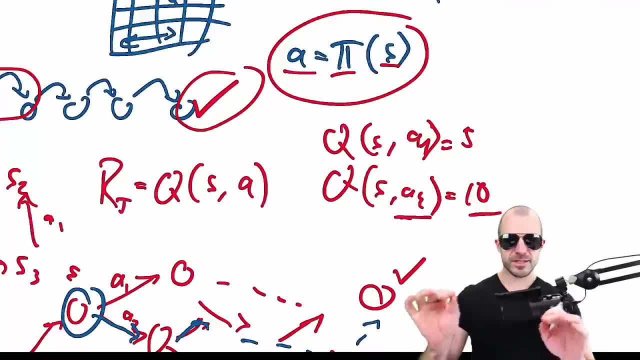 but the policy is simply: you could write it down, right, you could make a table and say: well, if you're in this state, do this. if you're in this state, do this. And there can be good policies. 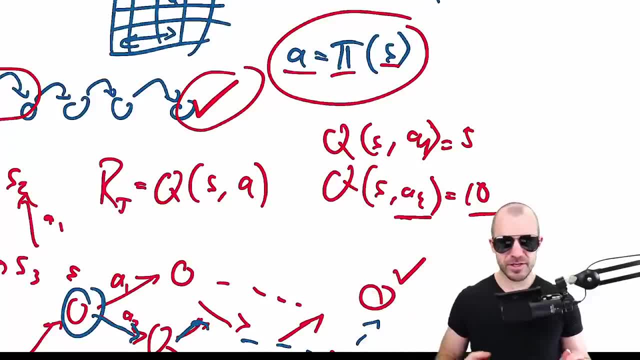 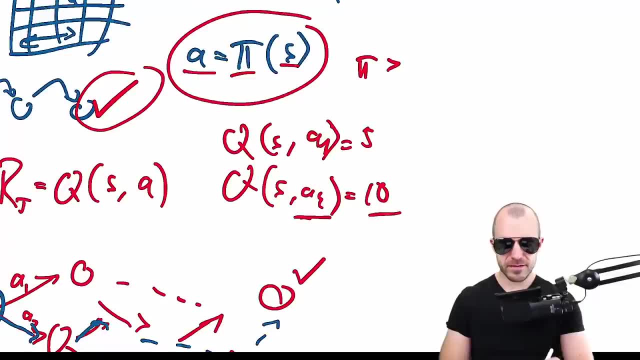 which lead to high reward, and there could be bad policies which lead to low reward. In fact, policies can be kind of ordered So you can say you know a policy is better than policy one is better than policy two If in any state you can be in the actions. if you follow policy one you get. 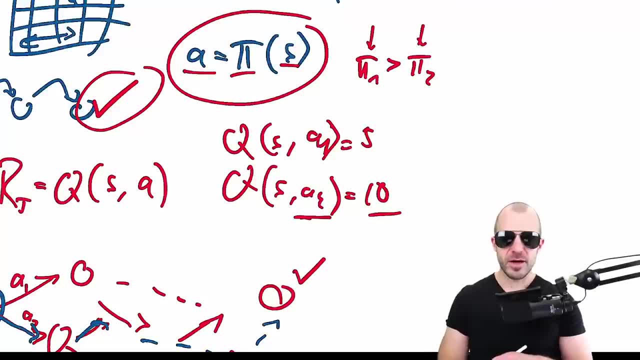 a better result. So you can say: well, if you're in this state, do this. if you're in this state, do better reward than if you follow policy two. But obviously these are not, that's not a total ordering in that sense, Because for some it can really depend on the state, But nevermind. So I 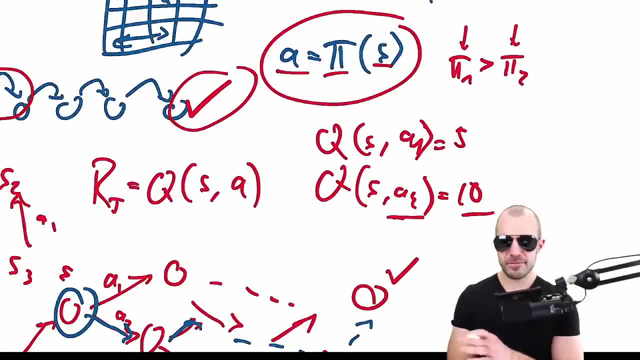 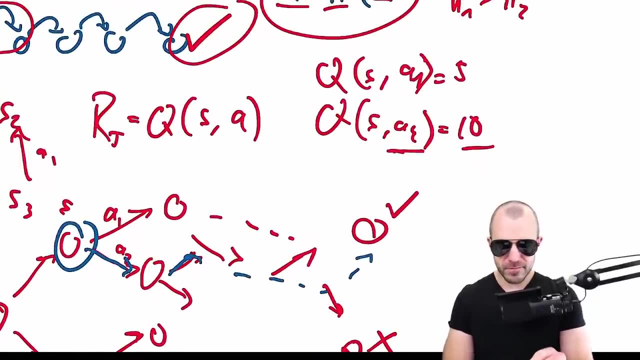 hope you realize the difference between a policy. a policy is simply a function that tells you what to do, And there can be good policies and bad policies. And the Q, the Q function. Now we can fully define it. So in order to fully define a Q function, I would have to also supply it with a policy. So usually, 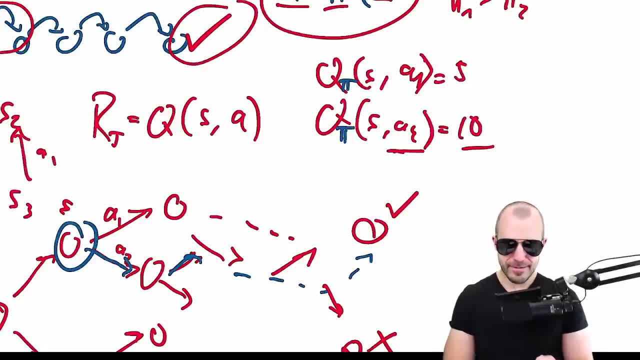 you say this, so Q, Q pi of s and a one tells you you're in, you're in state s. If you were to now take action- a one in this state and after that do whatever the policy pi tells you to do, then you would get a reward of five. However, if you're in the state now and do, 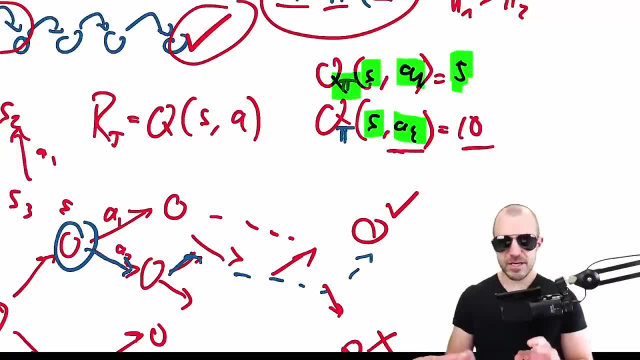 action two, and after that, equally, just do what policy pi tells you to do. then you would be in in a reward of 10.. So in a sense that what the Q function tells us is that we'll commit to following a particular policy. 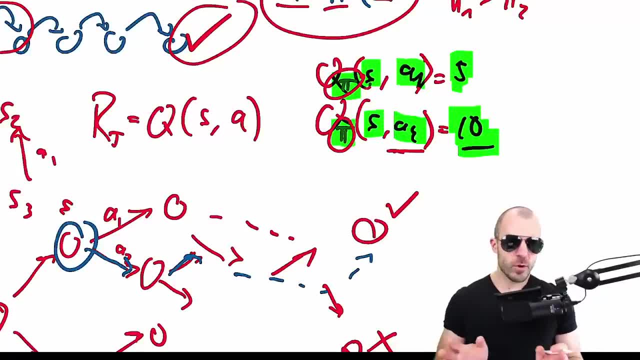 After this step. but for this step we don't really know what to do. So we plug each action into the Q function, say well, after this step I'm going to follow this policy right here, But please tell me what to do right now. And the Q function evaluates each action and tells you a reward that it thinks. 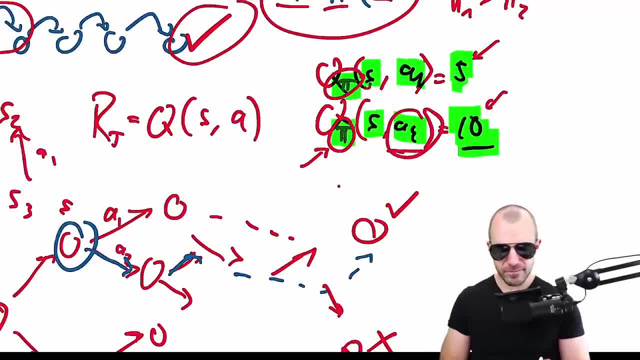 you know, after taking this action now and then following the policy we will, the total reward you'll get until the end of the episode. By the way, we haven't really specified reward and episodes right now, So in classic reinforcement learning. 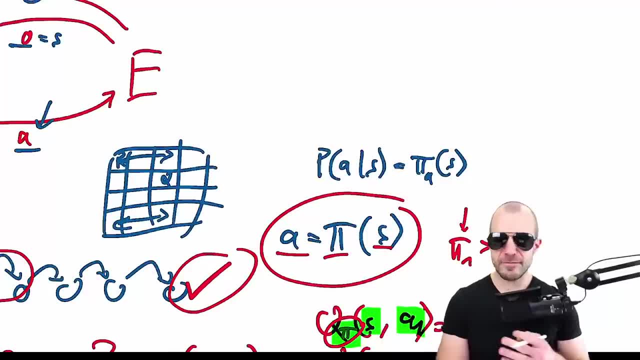 you always kind of assume that the episodes go for an infinite time horizon. So your total reward is going to be the reward that you get at step one, plus the reward you get at step two, plus the reward you'll get at step three and so on. Now you can see that if this goes on for an 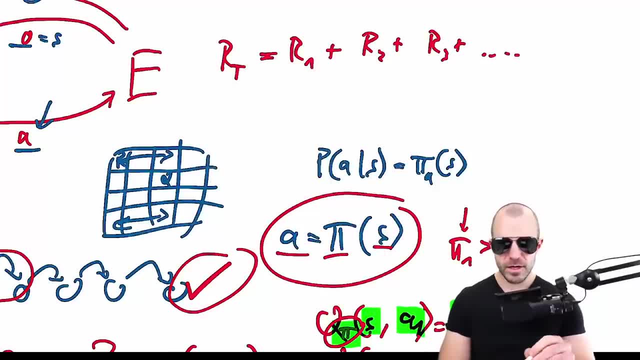 infinitely long amount of time, you can see that the total reward is going to be the reward that you get at step three, at step four, at step five. And so what do we do? OK, so we can say: well, the final we can say is if, in case of the, if we model it like this, okay, we can get infinite. 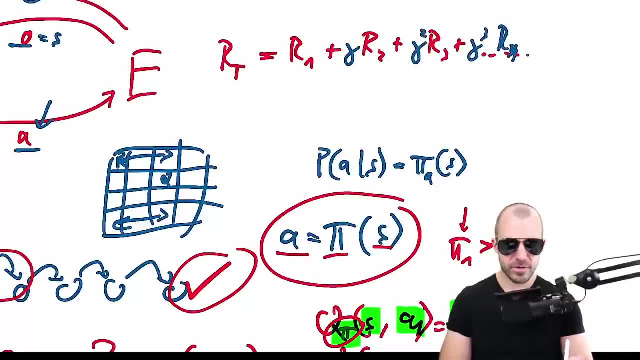 reward. So what people do, even in the finite case, is people say there's a discount factor, So plus gamma, three r3, or four. so So well, okay, I kind of screwed up my indices here, But we'll. 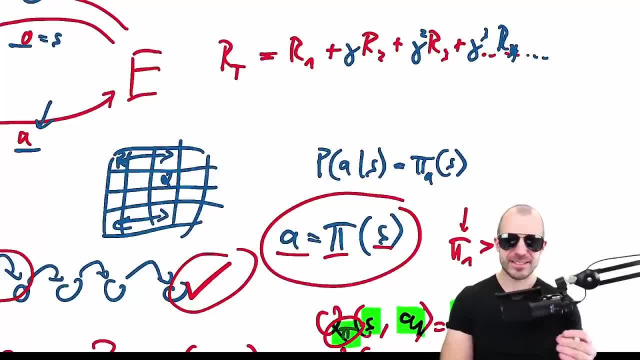 essentially say: you know, as time progresses, you know if I- and that's similar to how humans perceive reward- I guess if it's further in the future it's worth less to me now. okay, it's going to be worth more in the future, obviously. 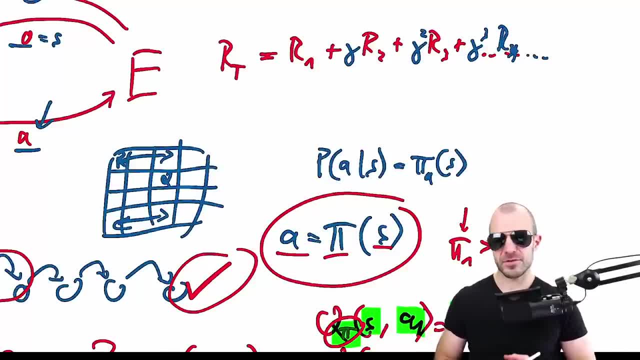 but it's worth less to me now. if you promise me $100 tomorrow, then if you just give me $100 right now- and that's not because I'm unsure about the tomorrow right, It's just because I'd like to have it right now- We can. there are other discount factors that model, things like. 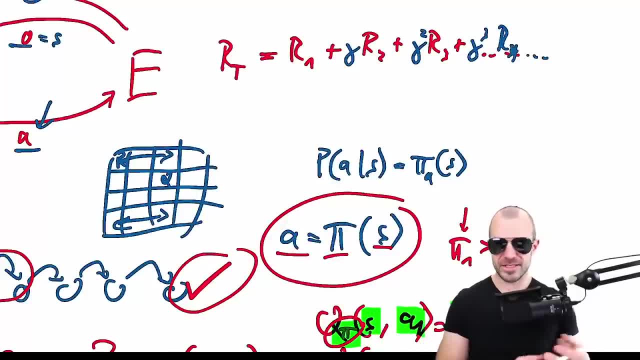 uncertainty, either in the problem or in our estimation of it. But the basic basics, basic total reward, can be calculated as a sum, And here I'm going to switch my, switch, my indices of gamma to the I, so I goes from zero to possibly infinity or T of the reward I'm going to get in that. 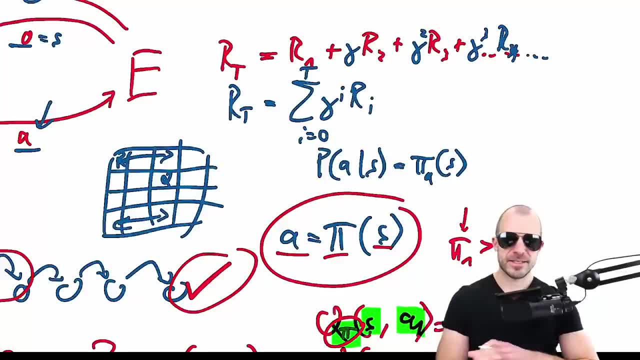 particular step. Okay, so this, this reward here is what I want: to maximize the total reward across the episode. And, as we said, if, if this here, if our episodes are such like in chess that just once, at the very end, I'm going to get a reward, we might as well set the discount factor. 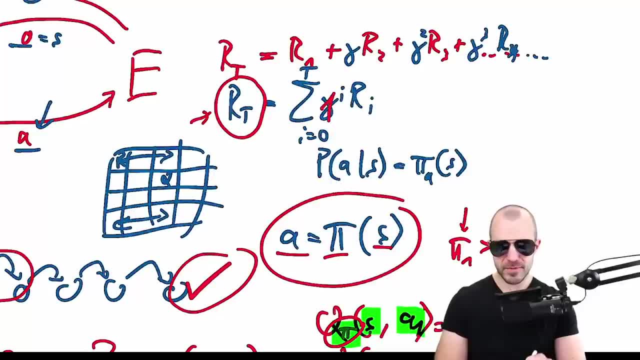 here to just one, And because it's this is going to unroll to just the, the last reward anyway. so, uh, actually, i to t. so this is going to, this is going to be reward r. i equals t, something like this. this is not super well written, is it, um? but you hope you understand what i mean. so 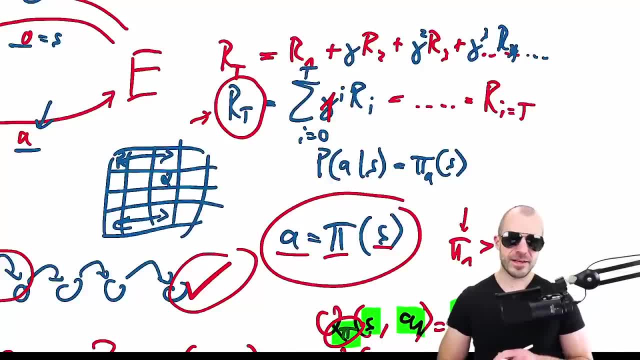 if we only get one reward, we might as well. and we don't care how long the episodes are right in chess, don't care how long a game is, if i win, i win, doesn't matter if it's in 20 or in 60 moves. we might as well put the discount factor to one and just take the last reward. 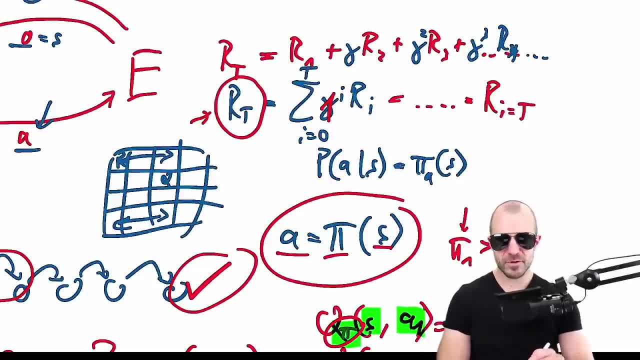 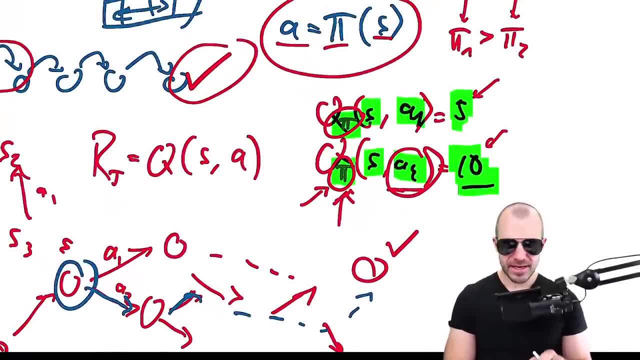 um, but in normal regular reinforcement learning there's discount factor. so why i did that? it's important to understand, uh, the the framing of the q function, and you can see that the q function is a little bit different from the q function. we could ask ourselves, why is this 5 and this 10? right? picture yourself: you're on a chess board. 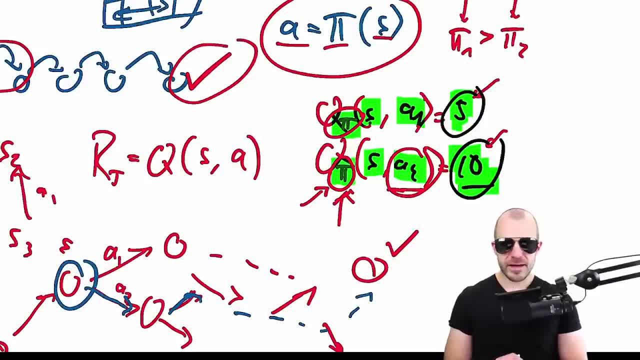 right and you have only two moves available and you ask the q function, you tell the q function, okay, i'm gonna. i have like, i have like, uh, i don't know, i have like gary kasparov on the phone or carlson, and i'm gonna, i i can call him after this move. right, so that i'm gonna. this is the. 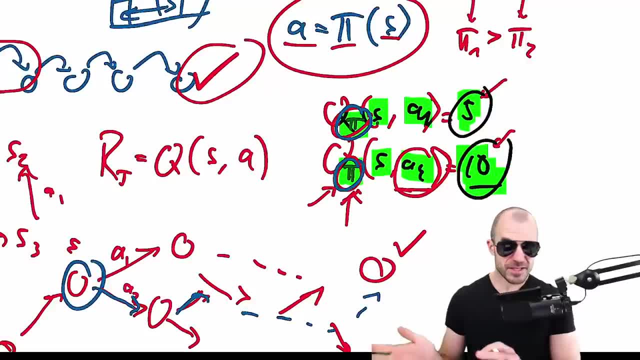 this is like a good policy, i know, but i just need to know what i have to do in this particular move right now. after that, i'm gonna call magnus carlson and and he's gonna tell me whatever to to do. but you know how? should i move my rook, or should i move my queen? and the q function is going to. 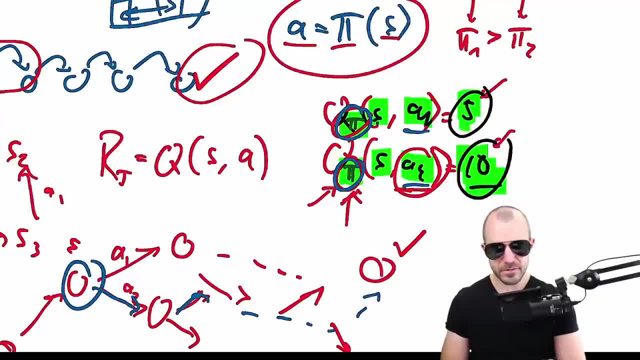 tell you: well, if you move your rook- uh, you're even if you call magnus carlson after that, your total reward is going to be five. but if you move your queen right now and then call magnus carlson, your total reward is going to be 10.. 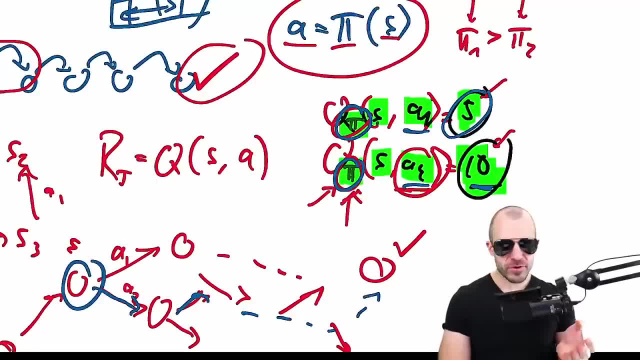 why it's important to understand the reason why these numbers could be different, and there could be two reasons. reason one, which is probably what you're thinking first, is that, well, the current action of moving the queen just gives me a higher reward, right, just um, actually chess isn't really. 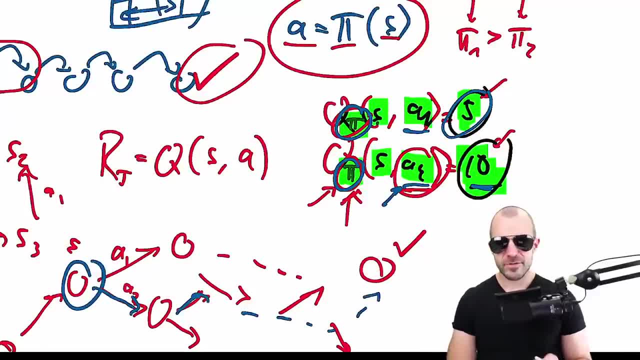 good example for this. so it could be that in a reinforcement learning problem, just the current action to it just gives you immediate five reward, right, and after that you'll go on, whereas action one gives you no reward right now and that's why it's five different. but there is another reason and that could. that's if you're. 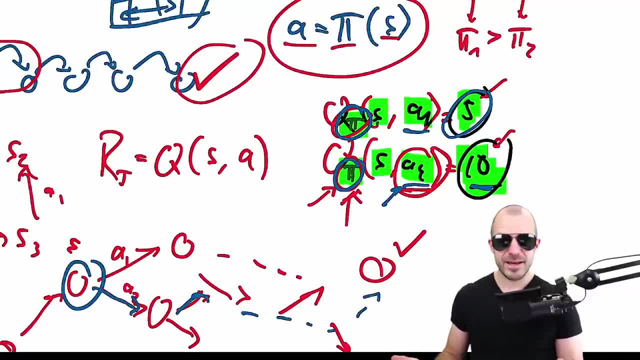 playing chess, then that, for sure, is the reason, namely, um, even though you're following the same policy after that, you will end up in a different state if you take the two actions. so if you take action one versus if you take action two, you'll be in a different starting state. 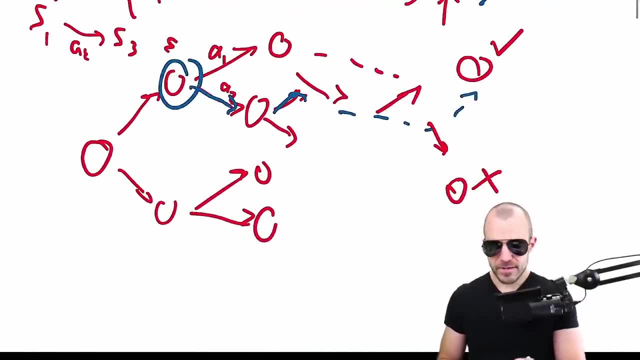 so if you're here, take action one, you'll be in this state, whereas if you take action two, you'll be in this state. now these actions could be on their own, relatively neutral, but because you're in a different state, you will have much less chances of ending up in a bad or a good state. 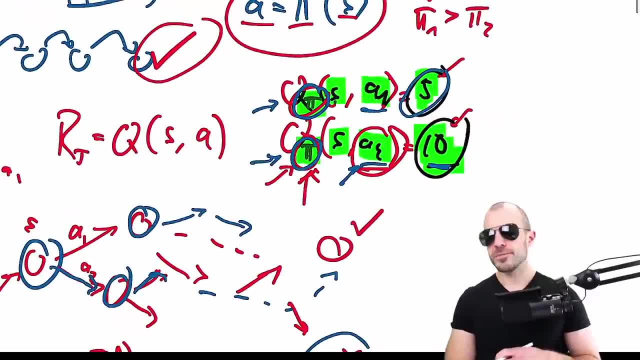 depending on the state you're in. so the q function encompasses both of those things like how good the current action is in the current step and also how good the current action is looking ahead in the state that you'll be in. and that's going to be lead us to the one of the 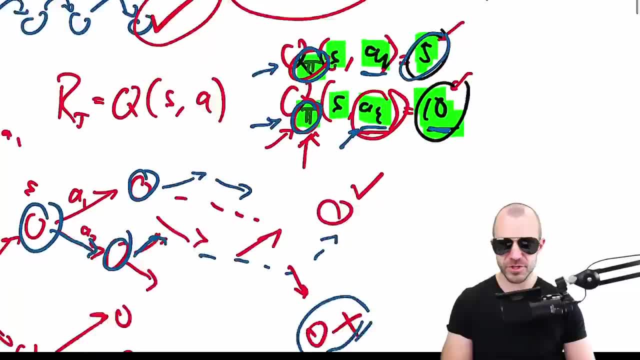 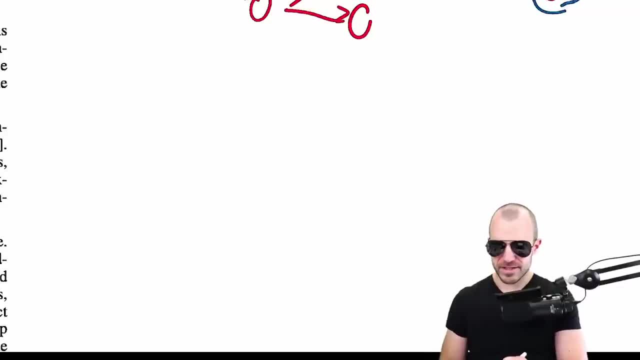 fundamental um equations, recurring equations in q learning, which is going to be development equation. the fundamental thing here is this: the q value in state s of action a and following policy i after. so after, the next step is: what's that going to be? well, that's going to be the reward. 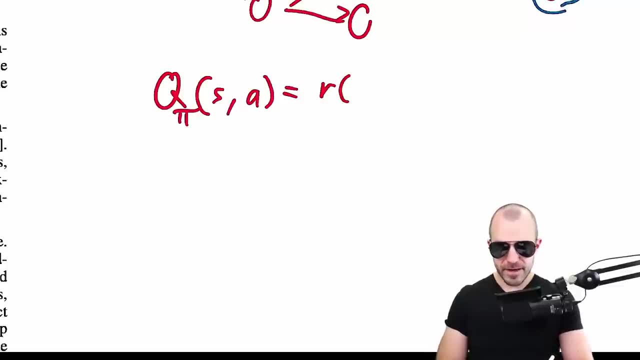 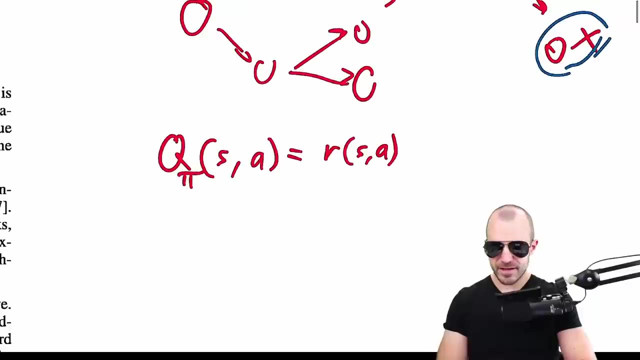 of performing action a in step, action, a in state s. so the immediate reward of that step, i think, before we've gone capital r, let's go lowercase r. so let's say let's say, like, capital, r is the total reward and that's going to be the sum of discounted lowercase r's. 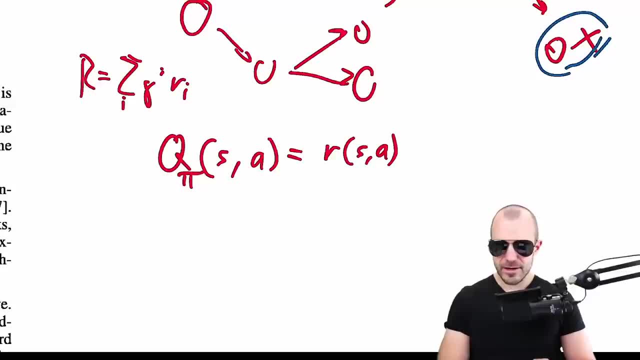 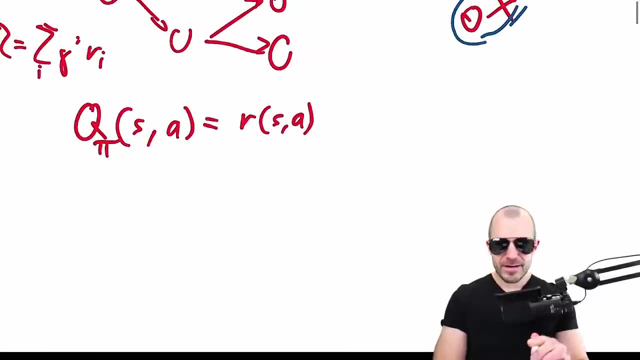 okay, and the lowercase r are the um rewards i get in the individual steps. okay, so the q value is going to be: what reward do i get in the immediate step that i'm taking, right? i'm gonna. maybe that's zero, right, but there in, there could be a reward right there if i put a checkmate. 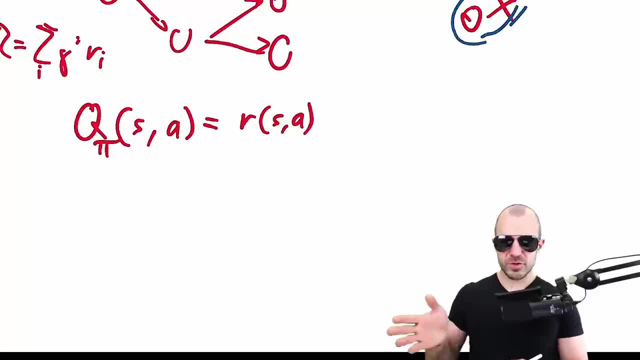 it's a one. if i am in doom and i shoot some monster, i do get actual points right. so this is reward. uh, note that there is no pi is not here, and that's because pi only matters after the next step, so that the the reward is only the current step plus whatever comes. whatever reward i'm going to make, 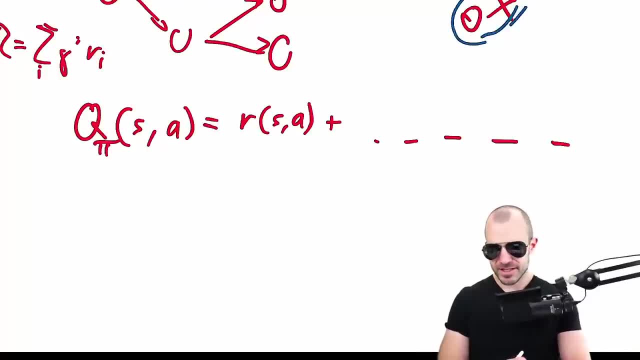 from the state that i end up. so let's just say: let's just say, if i'm in state s and i perform action a, i'm going to end up in state s prime we'll. we'll understand, or we'll understand, or maybe s prime a or something like this: we'll understand that. 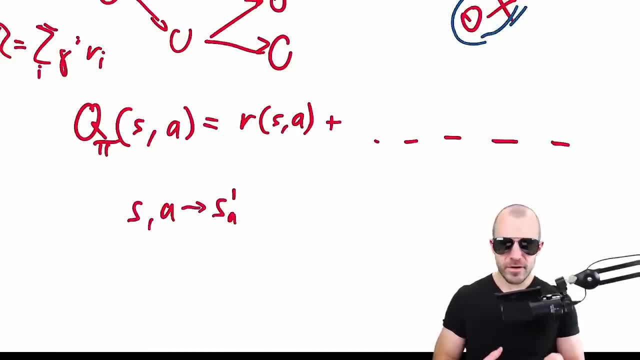 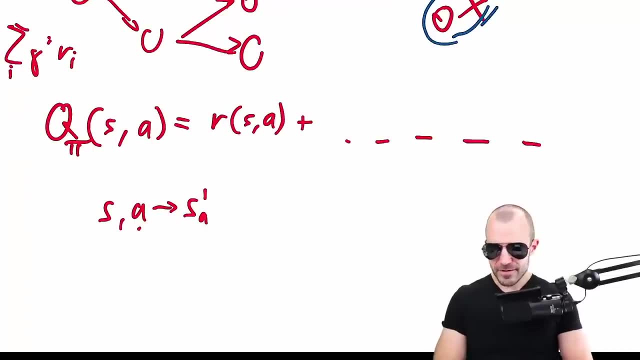 means the state that i'm going to end up with if i am in state s and take action a. so the reward that i'm going to end, that i'm going to achieve in the whole rest of the game, uh, from this state. well, what's that going to be? isn't that just going to be the reward? 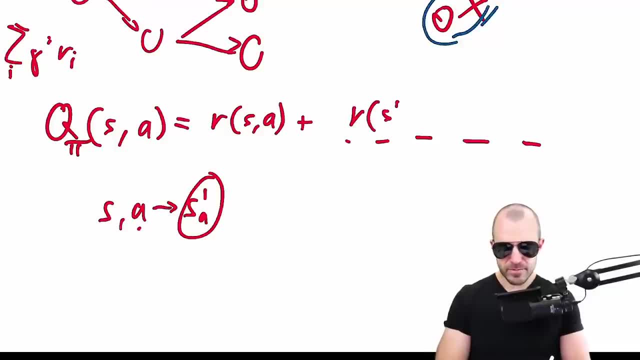 in s prime, you know. and then what action am i going to take here? um, i could say i can take the action whatever pi of s prime is going to tell me to do. and, uh, i'll do that for all the s like, for all the, for all the s primes that are coming up. i hope that's clear. so in the next step, 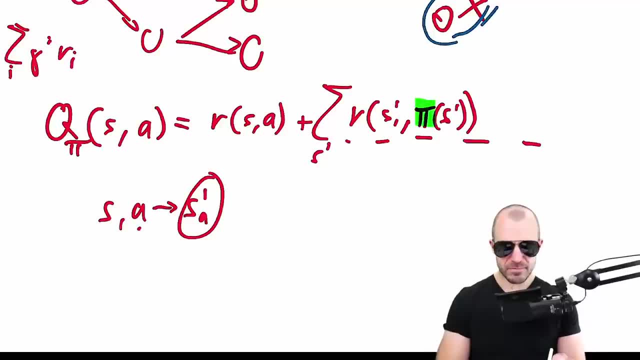 i'm going to just ask: well, what does pi tell me? um, what does, what does pi tell me to do? that's the action i'm going to take. i'm going to get some reward. i'm going to get into a new state. then i'm going to ask pi again: what action should i do? i'm going to take that action. i'm going to 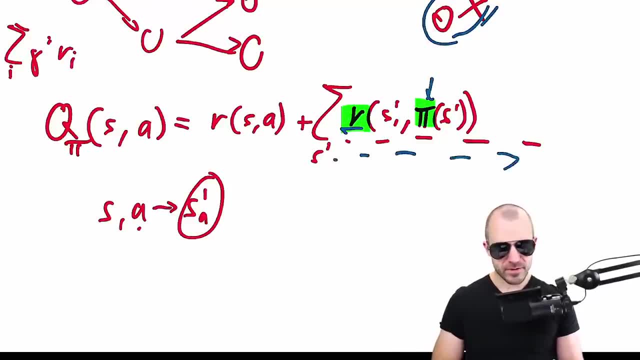 get some reward and so on. so this reward is going on until the end and we've split up our. we've split up our problem in two parts. the left part here is not dependent on that pi and the right part here is not dependent on the a right here. okay, now we can think of something and say: 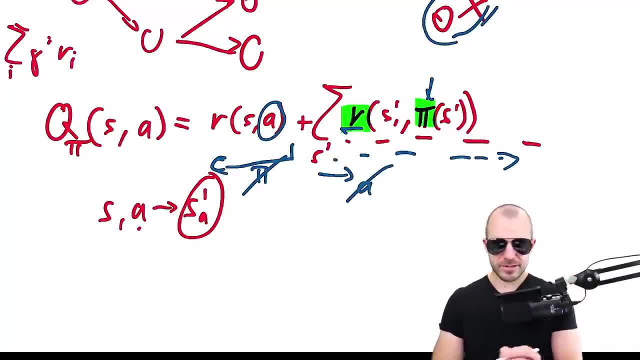 well actually here, sorry about the one apple pen confusion, this thing here. i just i just said, well, i have magnus carlson on the phone. why don't i just kind of call magnus carlson right now, right, and that's that's. that's one thing. okay, that would just solve the problem. the other thing: 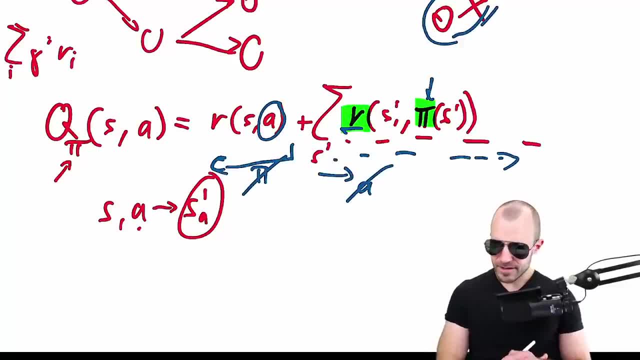 that i could do is i could say: well, if i have this q function available, if i have it available, if i can ask the q function, you know what? what should i do right now? to get like the best or to get the reward? to get like i can ask for a given action? what reward will i get across all? 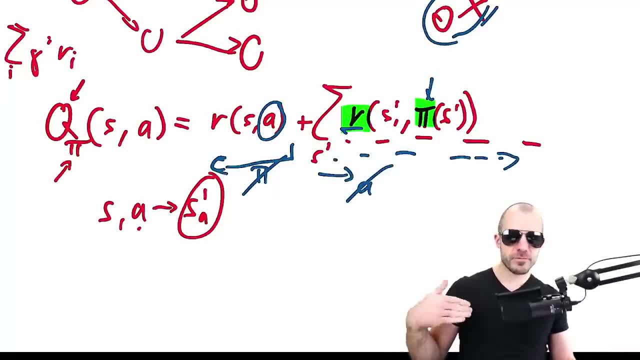 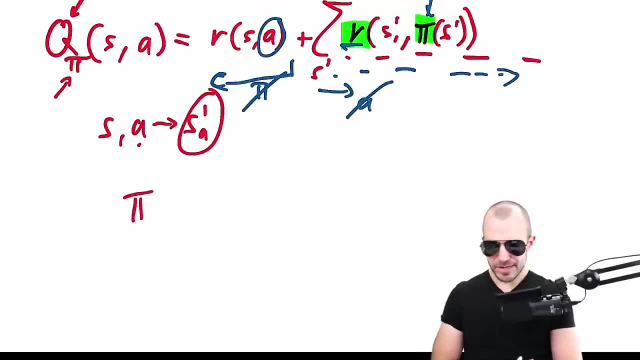 the game right for a given action right now, which means that i can define a policy policy and we're going to call that policy uh pi q for now, and the policy takes in a state and it's going to give me an action and i'm just going to say: how about? 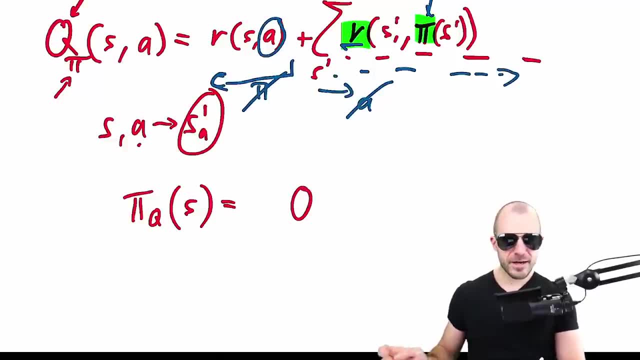 how about i just always, whatever state i'm in, i'm always going to ask my q function what to do, so and i'm always going to take whatever the maximum is right. i'm just going to plug every action into the q function and it's going to tell me a number and i will just do whatever. 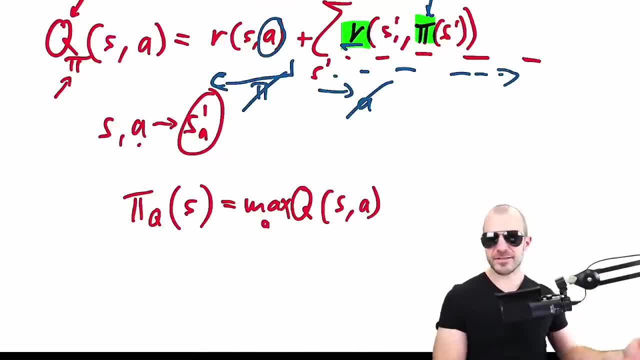 the highest, whatever action leads to the highest number, and that is a policy, right, that is, if i add every step, just do that, just do ask my q function. uh, that is a policy, because i can plug in a state and i will get out an action. now again, this q function is incomplete. we have to supply it a policy. and here is where. 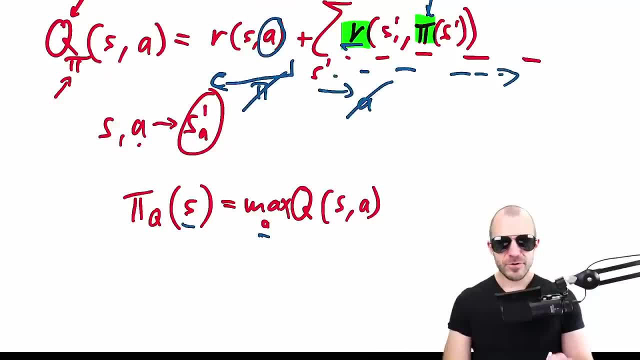 the recursion comes in, i'm going to tell the q function i'm going to what happens if i'm going to do action a right now and in the future. i'm going to act according to the policy where, in each step, i ask you q function what the best action is. so this it's. it sounds i'm making it. 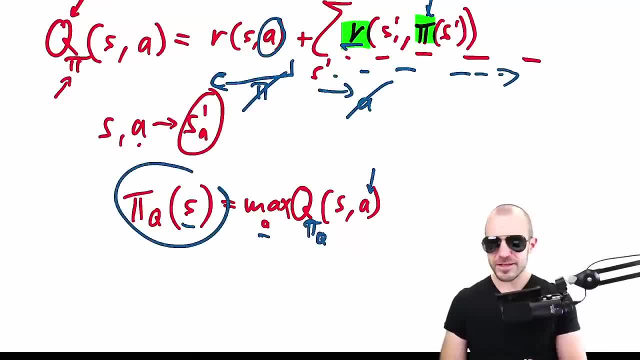 more complicated than it is, but essentially we're defining a policy that's defined itself by always asking the q function what i should do right now. if i intend to follow the q function also in the future and if the q function is actually good, then that is going to be the the optimal policy. 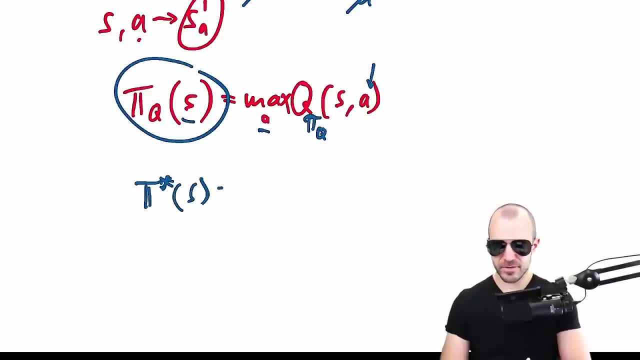 so we call it like a q star of s is going to be. i'll always select the maximum, the maximum action according to my q function um, by following the optimal policy. after i did that, and that is called development equation um, and it gives us hints on how we can learn these things. now you have to. 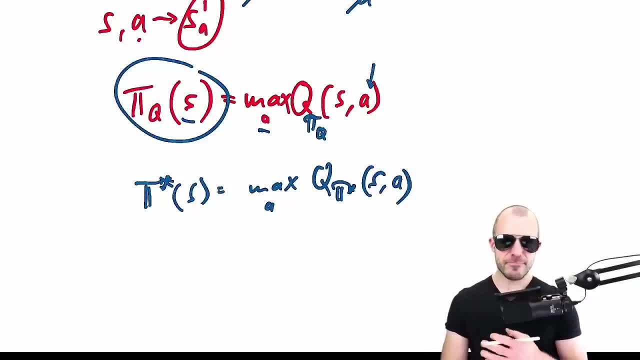 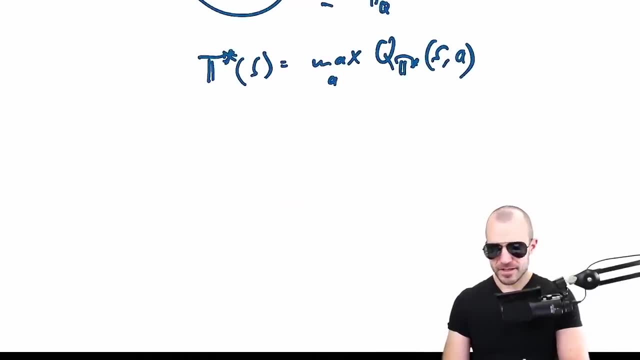 imagine q learning. it can be done in many, many different ways, but essentially what it boils down to is the following: so i am in a state s i ask my q function, hey, max, a okay of q s a ask that it's going to give me an action. actually. 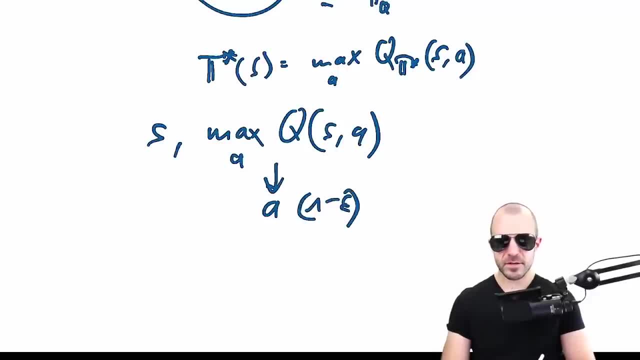 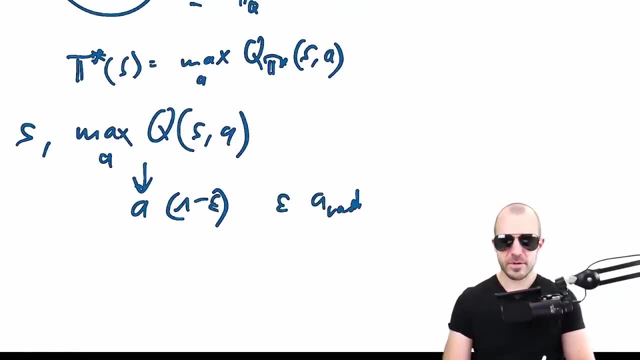 i'm only going to do that with one minus epsilon amount of times and in epsilon amount of times i'm just going to take some, some kind of a, some kind of a random, random, random action, explore, exploit, right. sometimes i just want to do something else because i might not, might not be the best right now. so the q function, um, i don't have, i did not. 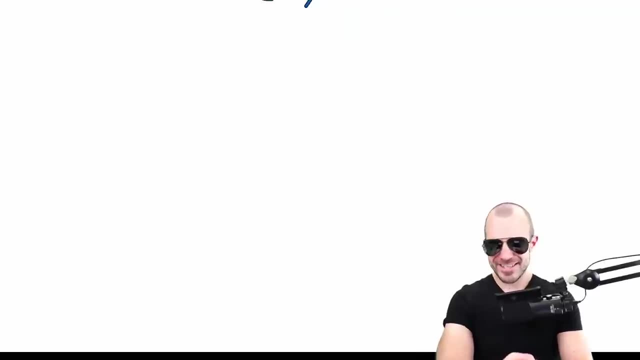 pull this up correctly. so imagine i don't have the q function now so far. we've always imagined we have this magical q function that just knows everything about our problem and can tell us accurately what will happen in the future. obviously, if i have that, i can just always ask it. you know which of these actions is the best one. 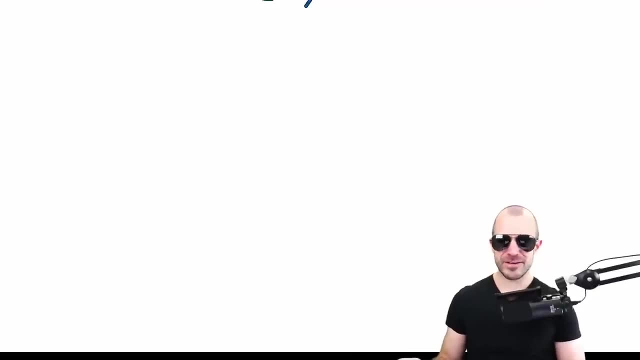 and that's precisely what we can't do if we don't know anything about the problem, and therefore q learning is all about. can we learn this q function? so the q function is now going to be parameterized somehow and it needs to take a state and an action and it has to tell me some sort of 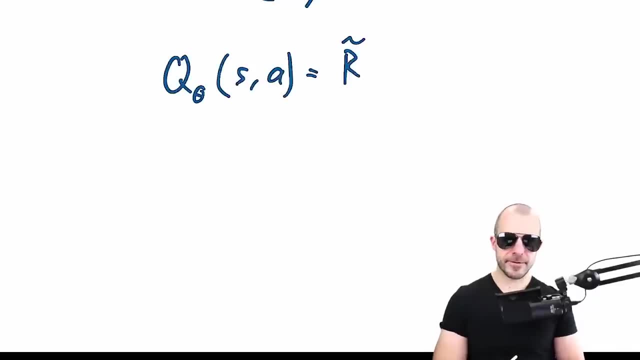 some sort of an estimate of r. okay, um, imagine, imagine i am in a reinforcement learning problem. right, i am here, my little figure is here and i ask: it goes this way. and there is, i don't know, it's the dinosaur game. then it's not a person, it's a dinosaur, is it? but let's say there is a bird coming at me and i ask: 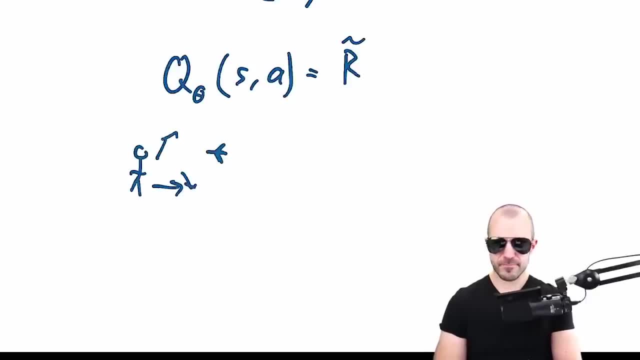 should i jump or should i duck right? and these are the two actions and let's say i choose either one. and i'm going to take this first step of the question, because the question is, of course, q learning, or the question is, of course, q learning, and q learning can be performed as far as i'm aware. 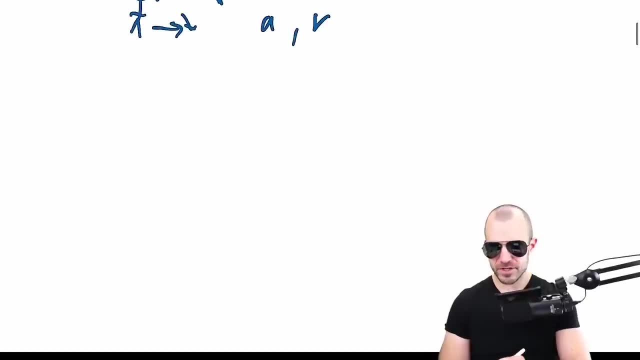 you don't always have to choose the maximum q. you can do a bit of exploration here. so you've actually performed some sort of action and you've gotten some sort of reward of that step. now what does the bellman equation tell us? the bellman equation tells us that the q of pi and q of the state s and action a 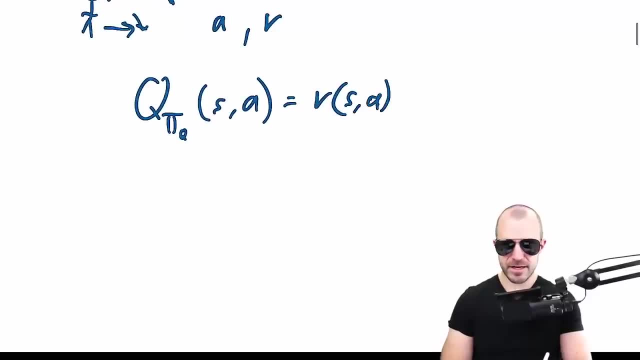 should be the reward i'm going to get: um in state s and action a plus the discounted future reward and that's going to be the discounted q value of q. did i discount over here? i probably did not. i probably did not discount over here um of being in s prime a. so i've done action a, i've gotten, i've, i've. that has led to reward r. 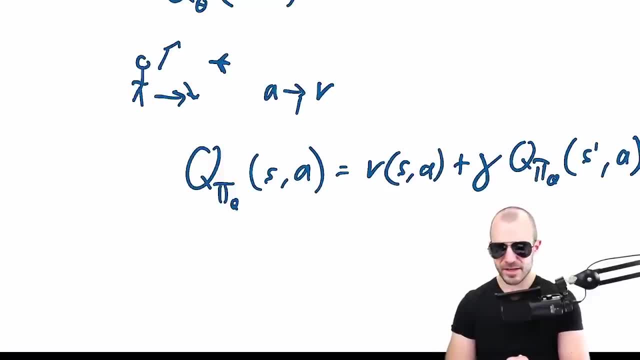 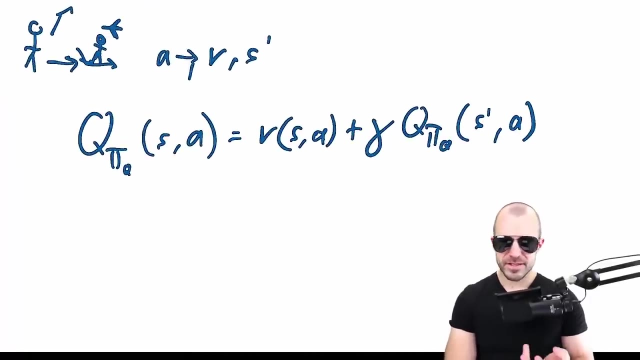 maybe reward is positive, because i i ducked, i got a little bit further and that gives me a few points and i've i'm in a new state s prime. the new state is: i'm ducked under here under the bird, okay. okay, now what i can do is: um, i can. 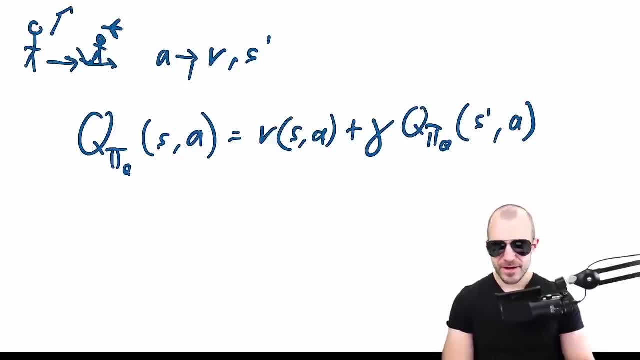 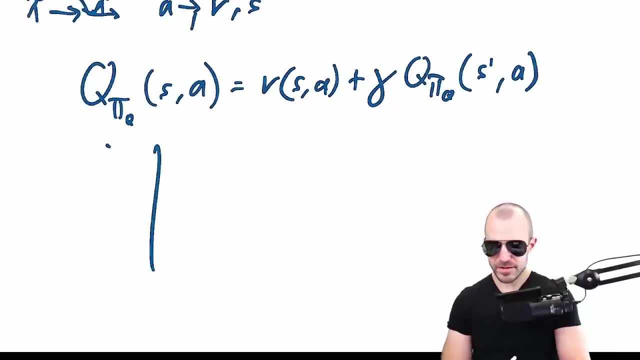 kind of self regress. so q learning can be done in multiple ways. the easiest thing is to have a table, literal table, that says that has the state s and the action a, so it tell. it would tell me: well, if you're in state one and do action one, then your q value is going to be five if you're in state one. 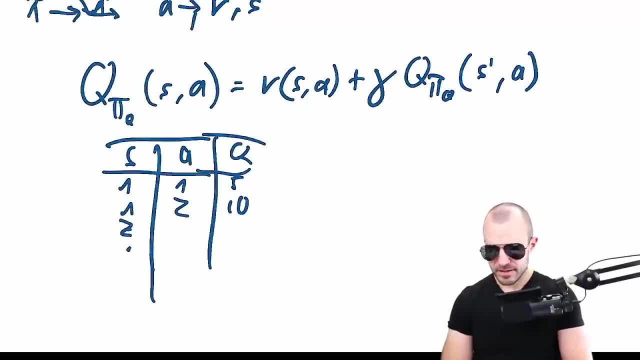 do action two, your q value is going to be ten. if you're in state two and do action one, your q value is going to be eight, and so and so on. okay, if we don't know anything yet, we'll just fill this here with random values. 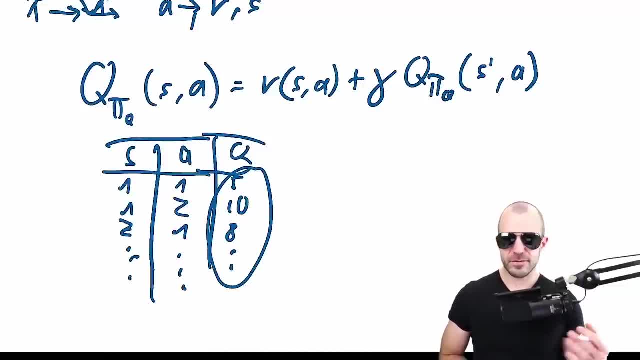 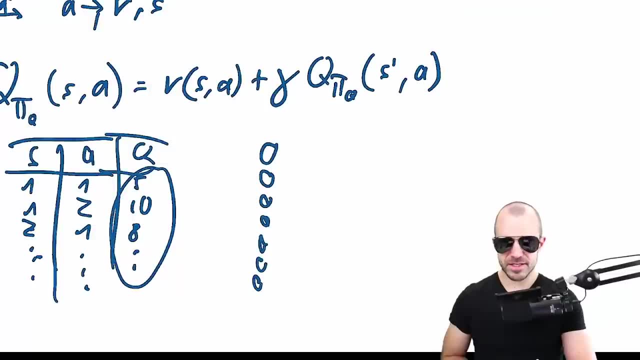 now there's obviously also a different method which you might be more used to, and that's: we'll build some sort of neural network. it takes in a representation of the state, so the state is going in as some sort of embedding or image. right here there's going to be some sort of a neural network. 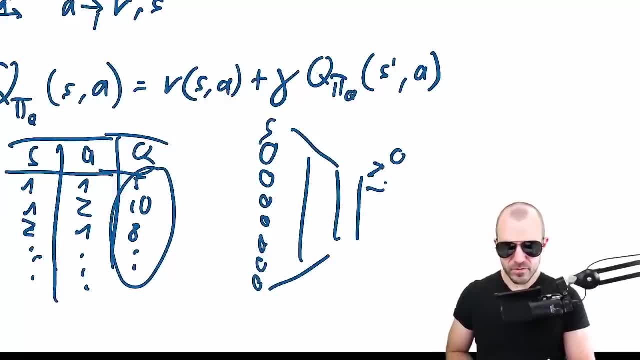 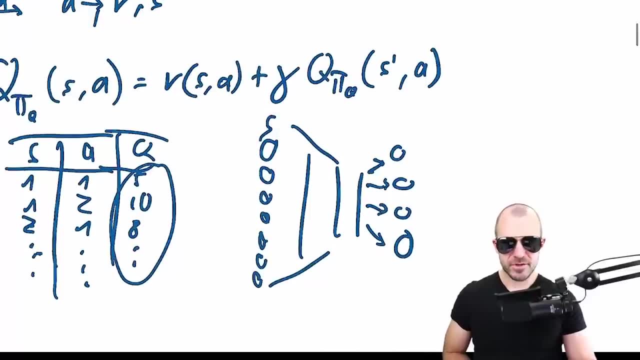 and then there's going to be one output for each of the pods, and then there's going to be one output for each of the pods, and then there's going to be one output for each of the possible actions, and then each of these is going to give you a value. there's also different methods. 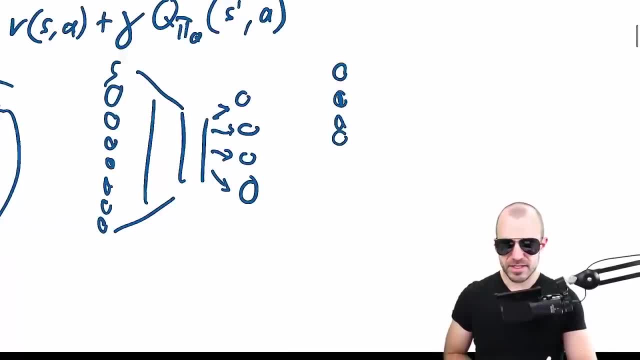 with neural network where you'll have as an input the state and you'll have actions also as an input encoded. so this part encodes the state and this part encodes the action, and the neural network is just going to give you one output, one number. however, you do it right, you have to initialize. 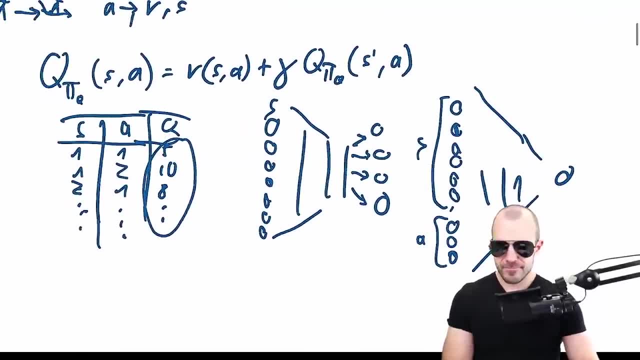 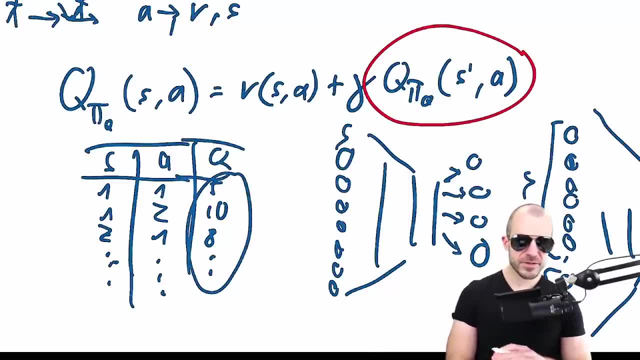 with kind of random numbers, and then what you'll do is you'll simply use your own estimate as a target. so you're essentially saying: well, whatever the q function is, um, if, if i ask it what the q value in this state is, given an an action, a right, it should. and actually this here on the right hand side isn't super correct. 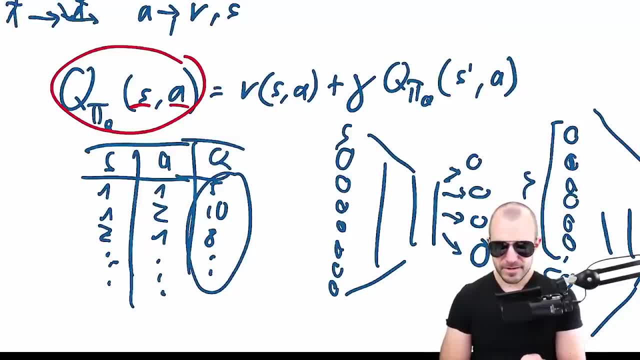 it should give me the. it should give me the same as if i take the reward i'm actually getting by doing this action, plus the future reward from the new state. now you'll see there's action, a here. action a actually needs to be marginalized across um action a needs to be marginalized across this policy. so this is: 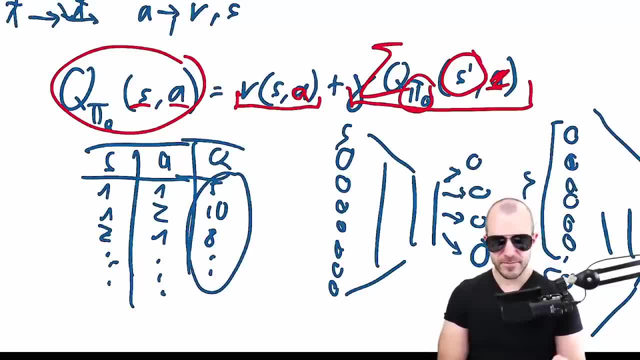 not action a from here um, but you can kind of see the basic principle. the q function needs to fulfill the fundamental recursion of bellman, which means that the q function in this state must somehow be the reward i'm getting by following the q function plus the q function from the next state onwards, and even if i don't, 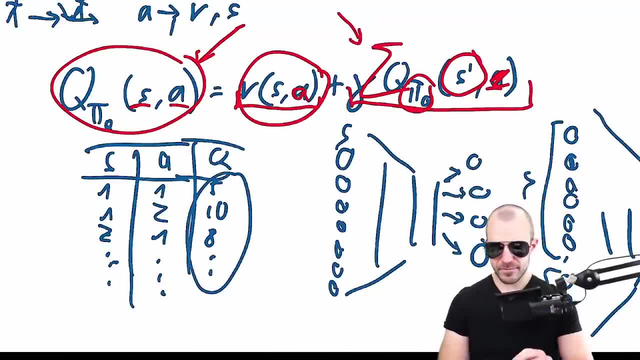 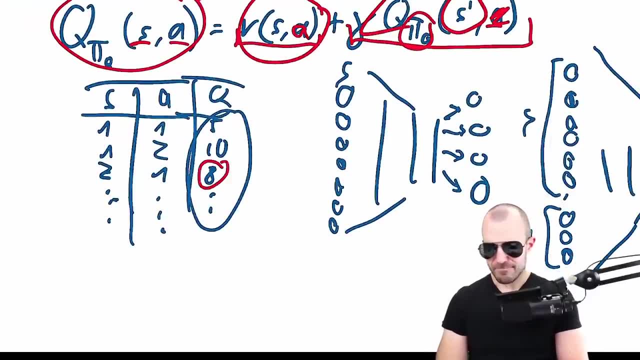 know the q function. yet i can kind of regress to myself. so i can, even if this is a crappy estimate as of right now, and i know if i'm in state one, i do this, i go here. that gave me a reward of maybe four. right then i know: aha, four and eight is probably 12.. so this here i really underestimated. 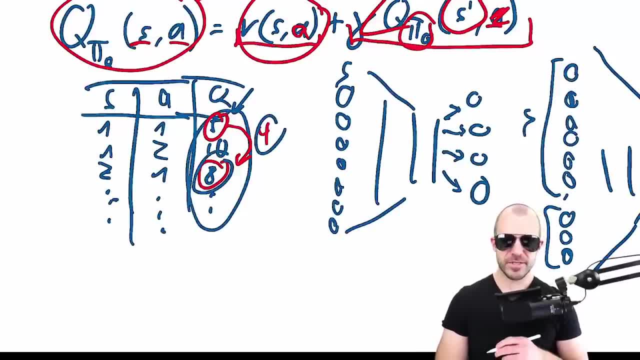 the total reward i'm going to get to at the end of the episode. so i should probably change that. i should make that 12 right and if we iterate and iterate we're going to get better and better estimates and should sort that might fluctuate and so on, and 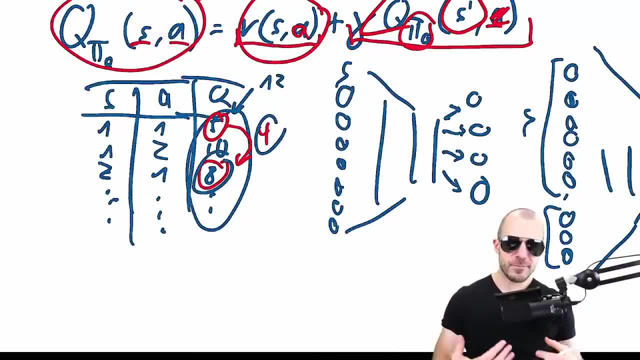 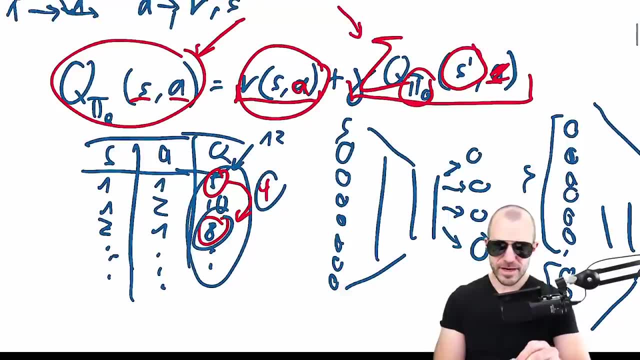 that's one of the problems of q learning. but you kind of taking your own estimates as targets and you combine them with the actual rewards that you get from the world. so you always say, well, the reward i'm getting plus what i estimate my future reward is, that's my target for the total. 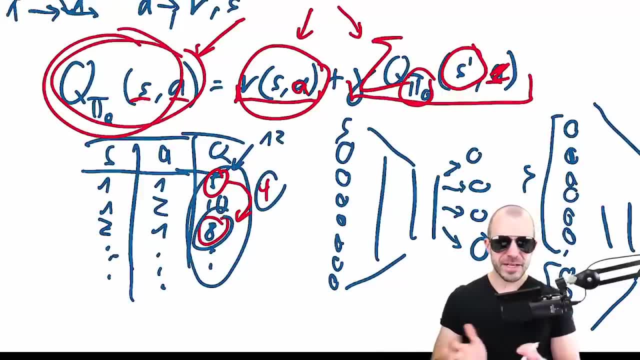 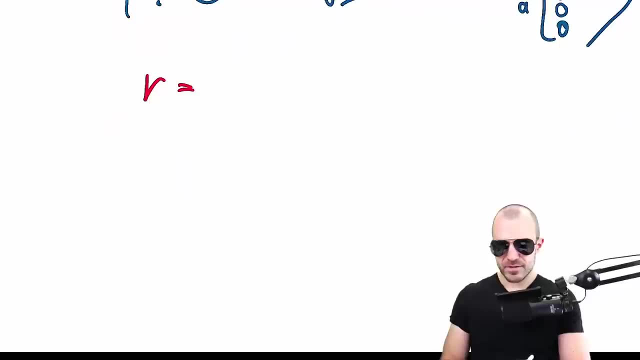 current reward, and thereby you can reduce the whole problem to just estimating single step. so the the single step is then the reward that you get from the world. that's a real number- needs to somehow be the q function in this state minus the q function in the next state. 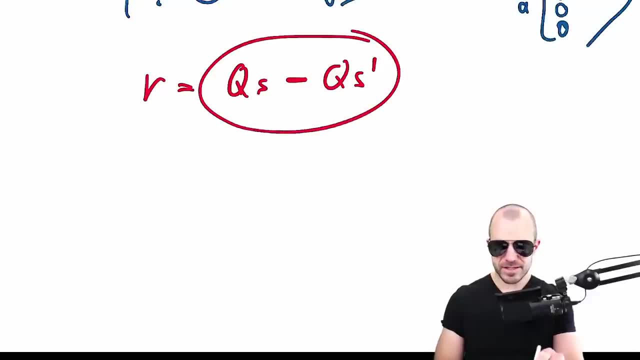 and you're going to train your q function so that this difference here matches the reward that you're getting. and you usually only train one of the parameters here and the other one you you kind of keep fixed, but i guess you could train both at the same time. i'm not sure that's super. 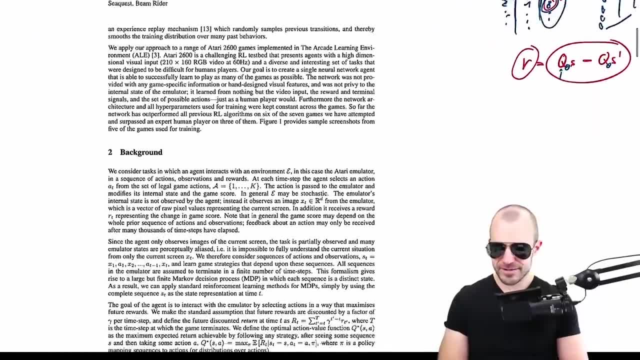 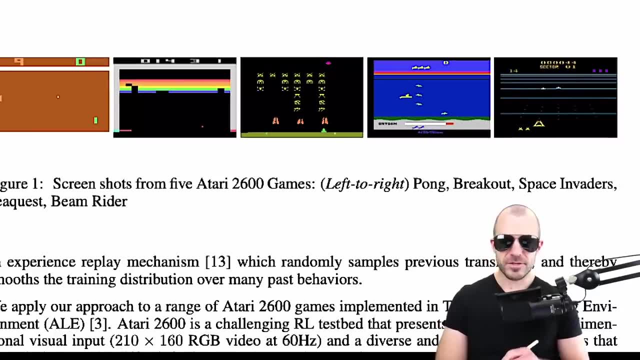 good idea and that's how we get to this paper. deep q learning considers atari games. so atari games lend themselves quite well to the combination of deep learning and q learning, because you have an input state which is quite complex, so you can't do the. 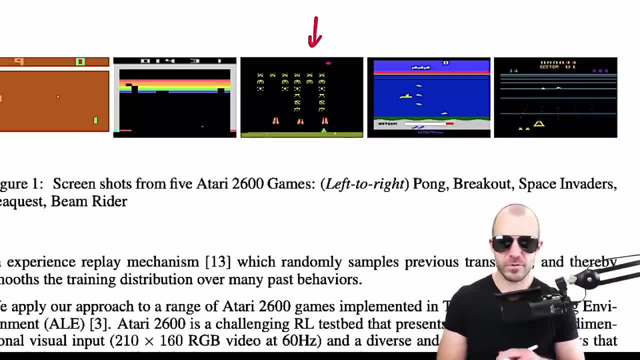 this with tabular q learning you have to do is with neural networks, so the input state is quite complex, lots of pixels and so on, but the output action space isn't that big. you can go like on an atari, you can go like left, right up down, press a button and that's kind of it. 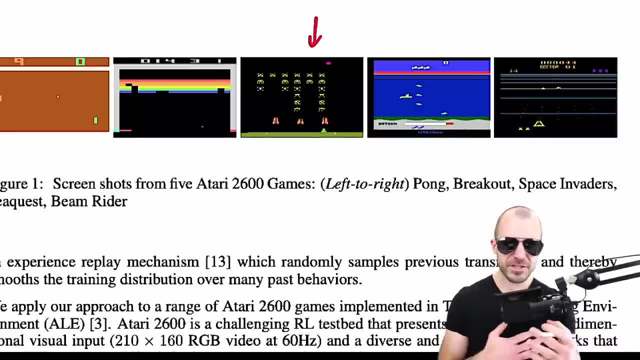 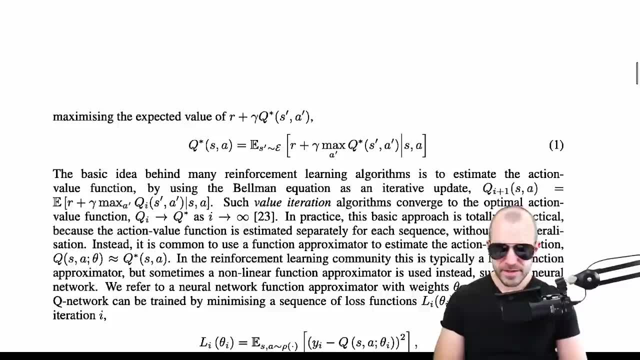 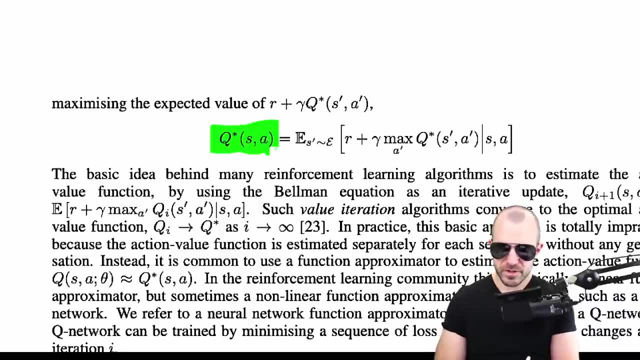 you have some combo actions of all of these, but the action space is very limited and thus they can actually do q learning right here. so you can see here the fundamental um equations that we've gone over. the q function with the star is the optimal. the q 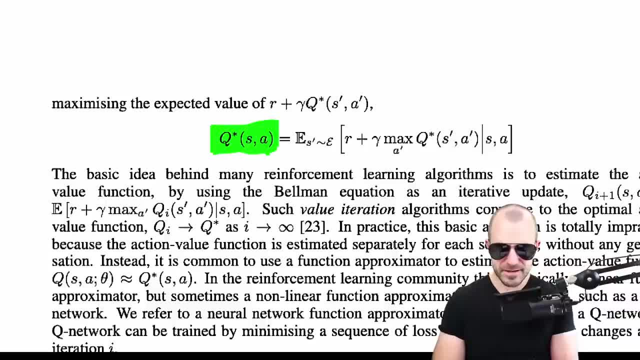 function following the optimal policy, that is, if i have my reward from the current step plus, if i follow the, if i follow the best action in the next step forward. okay, and this is the actual, correct way of working with deep learning. so that's how we get to the next step forward. 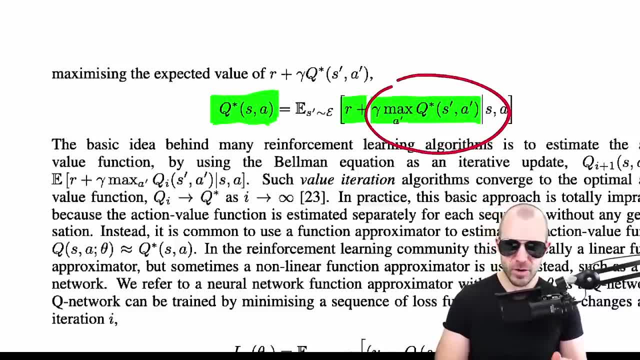 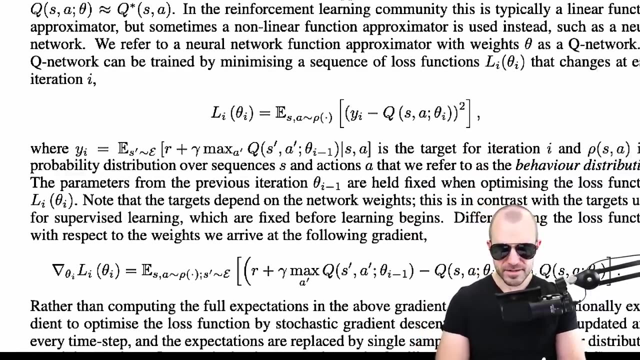 writing it right here. i botched that a little bit. i hope this becomes a bit clear now. so the the q function of the optimal policy is, whatever the reward. next step is plus the q function for the optimal policy. from the next step on out, here is their loss function. i said the loss function is y, i, y, i being maybe they. 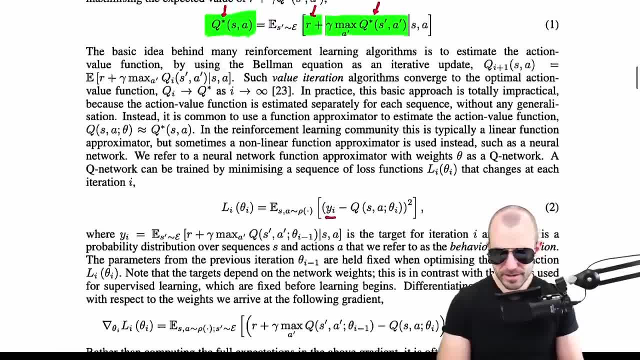 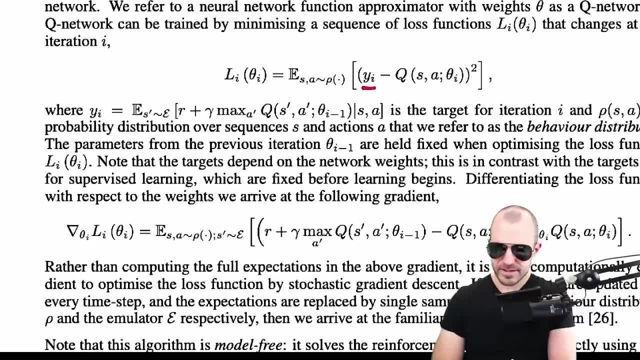 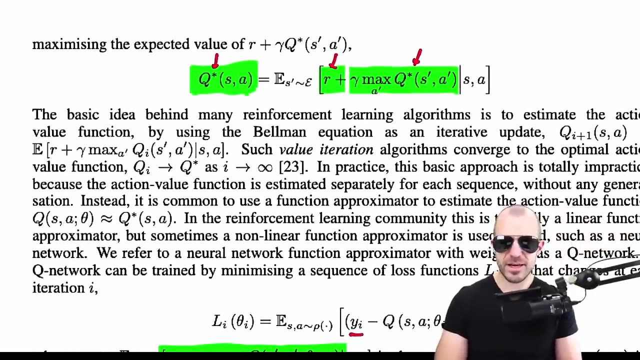 say that somewhere y i, let's see. ah, there we go where y i is. this plus this, so essentially what we, what we've just seen, so their, their target, their target is the right hand side here and um, so the right hand side must be equal to the left hand side, bellman says, for the optimal policy. this must be true and therefore, why don't we? 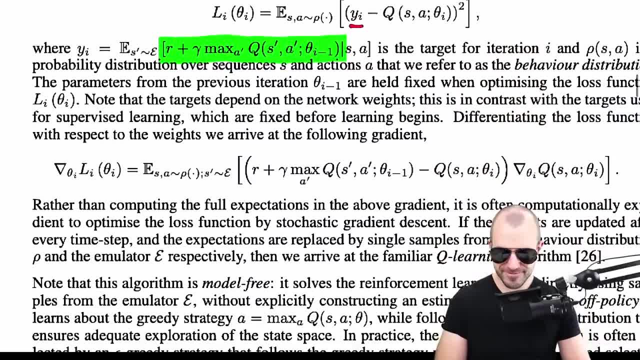 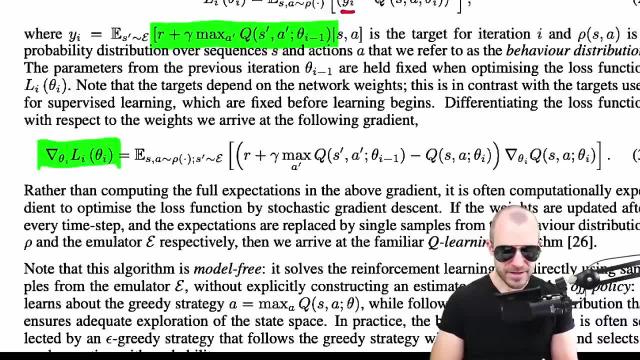 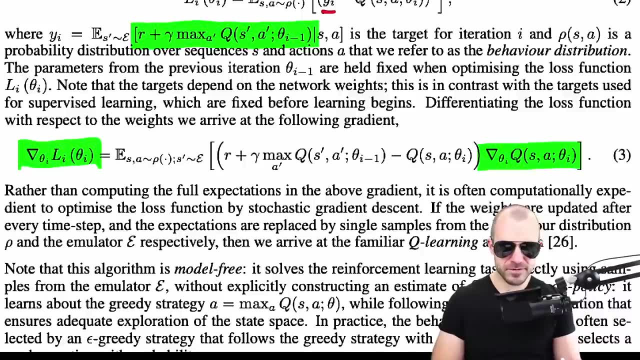 make it true using gradient descent. so the gradient they consider here gradient of the loss function is going to be. you differentiate through the q function of the current state. you keep the q function of the next state fixed. the reward is fixed anyway. so therefore you're going to take whatever you. 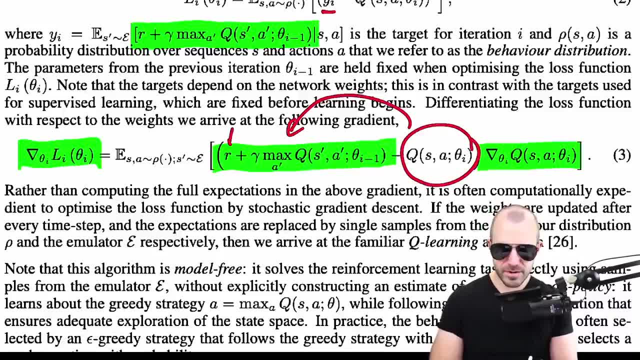 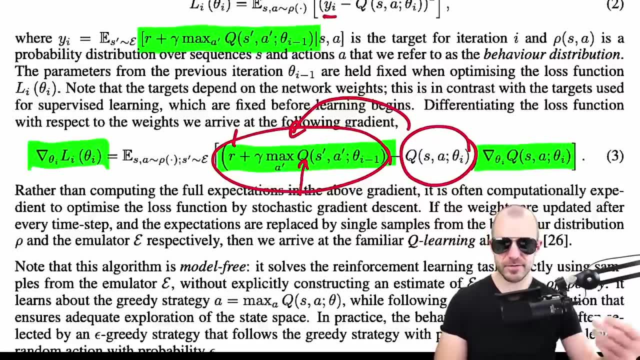 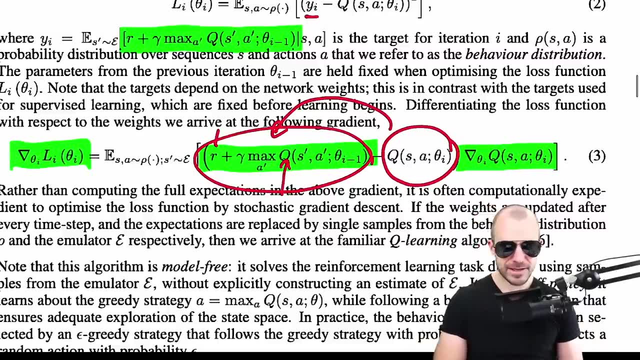 estimate currently and make it closer to whatever it should be. and again, that includes your own estimate of the future, and that's why it's a little bit different than like supervised learning or or something like this. so if we think of this in language modeling, right, you always have you. 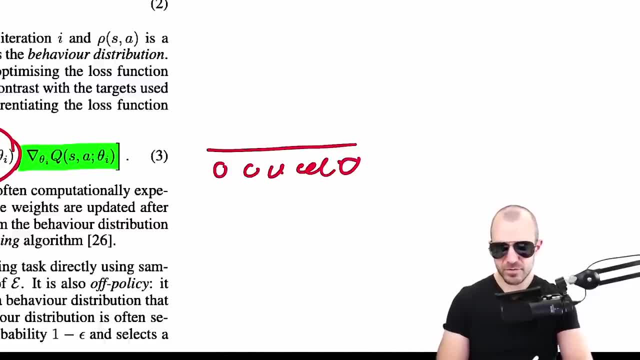 have a sequence of tokens and if you do autoregressive language modeling, then for each, for each token that you output- i will start one later- you actually have a target in mind. so, from here, you predict this, but you have a target. and then, from these two, you predict this one, but you have a target, and that's why you can do. 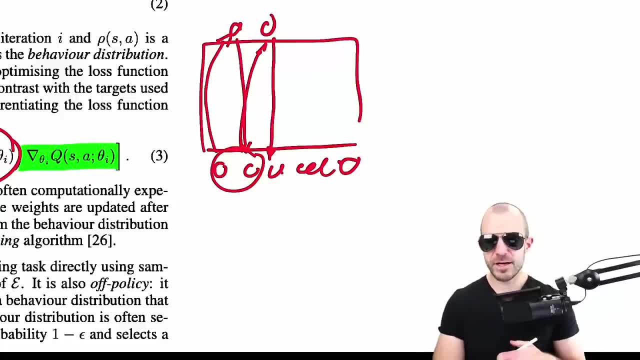 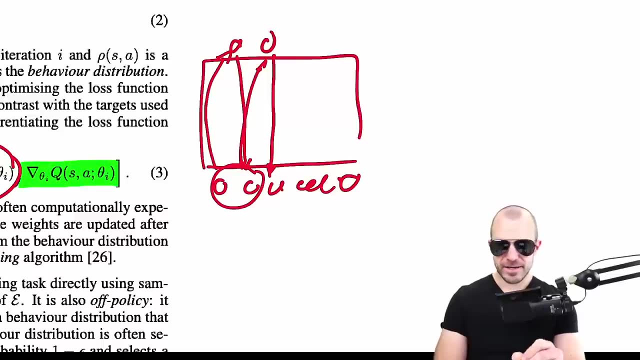 supervised learning when you do autoregressive language modeling, because you always predict the next token and that's a defined next token and that's either correct or not correct. if we talk about reinforcement learning in language modeling, it's more like where the whole sequence is going to be predicted first and maybe at the end you're 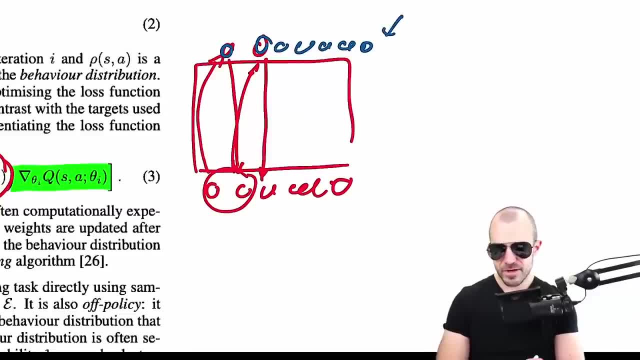 going to get some reward and then you need to figure out, well, which of the tokens actually were- the good ones, the bad ones, and so on. what you should do next, and that's where, currently in rlhf, proximal policy optimization is used. but it could be conceivable that q learning can be used. 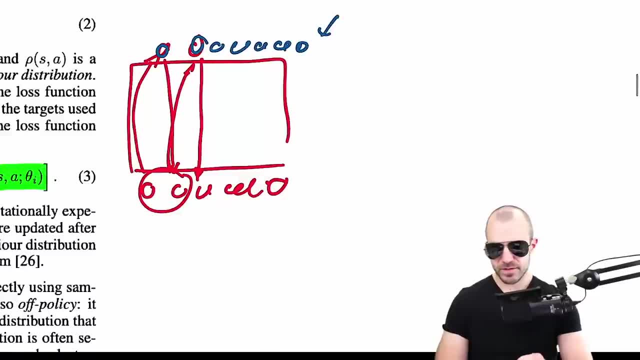 as well, because in language modeling we have a sequence, or rather a sequence of tokens that are, or a partial sequence. that's the input, and we can encode those really efficiently using transformers, and we have a fixed set of outputs, namely our token vocabulary, even though that's 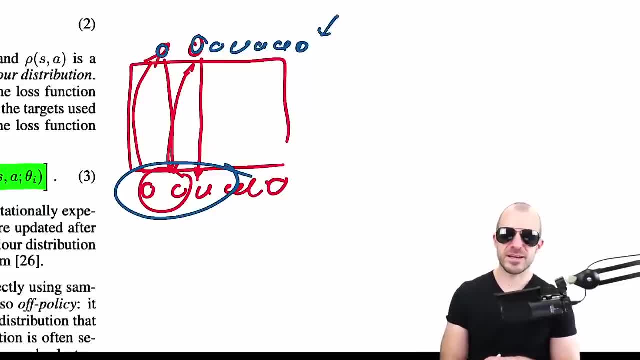 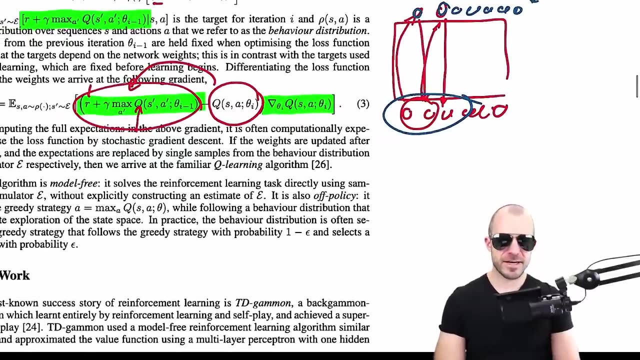 quite a big set of outputs. we have a fixed set of outputs being the token vocabulary that that defines, defines our action space. so to say so, q learning is not too, you know, too too far out there, except that with such um high action spaces, it, in my understanding, 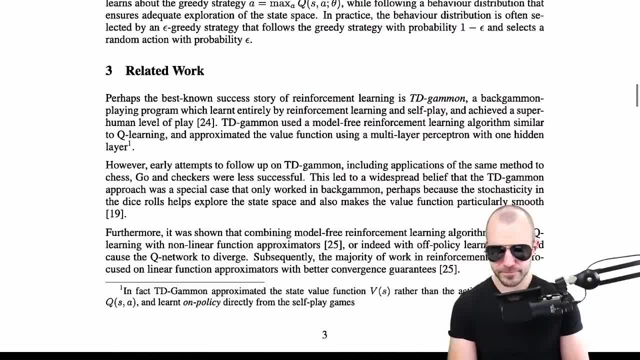 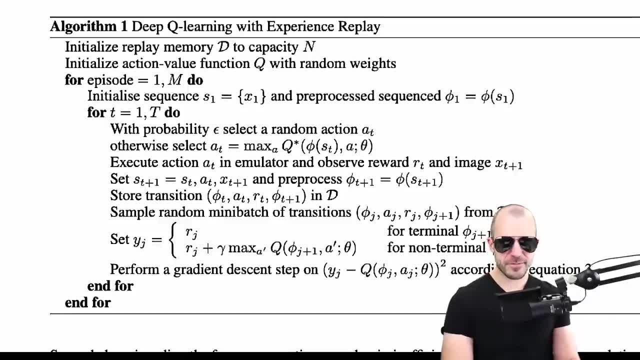 it tends to become a little bit brittle. let's just quickly go through what what they do right here. they have a few tricks up their sleeve. one is this: experience replay. so they don't just always learn on policy, but they have a bit of a buffer of things they do. 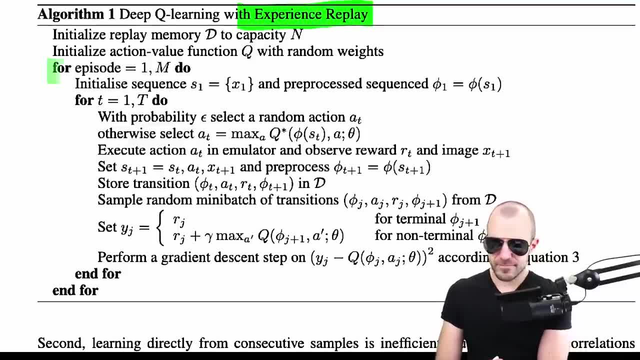 so in deep q learning for atari, they uh two episodes. they, with probability epsilon, select a random action. otherwise select an action according to the maximum of the current estimate of the queue function. again, we don't have it, we need to learn it. so at the beginning it's going to be crap, but as we go on it's going to improve and 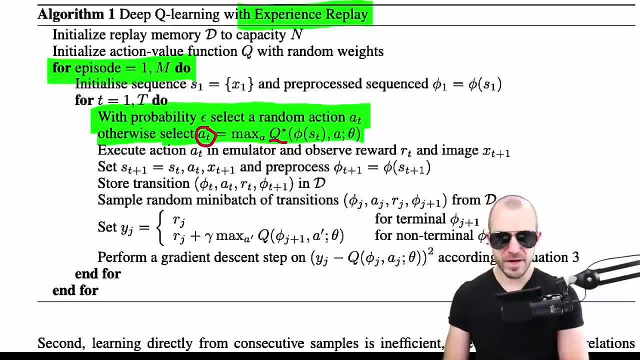 improve and improve, and thus we're going to play better and better and better games, which leads into states where we can explore more and more the good paths. right, and if we just explore the good paths, then, um yeah, technically we could explore everything. right, technically we could. 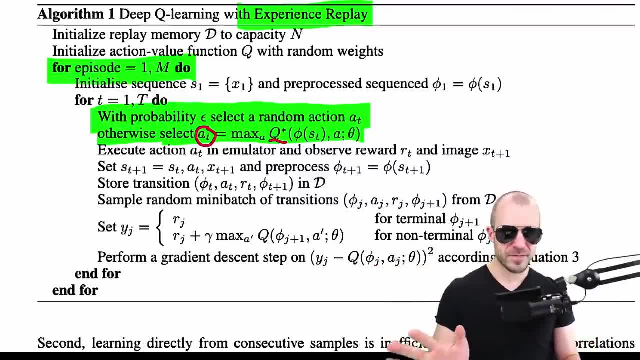 just run a random exploration in this environment and then learn from that. however, however, um, that tends to not be too good as long as- like, as long as these states are really big. so if there are many, many, many states, we don't just want to do a random. 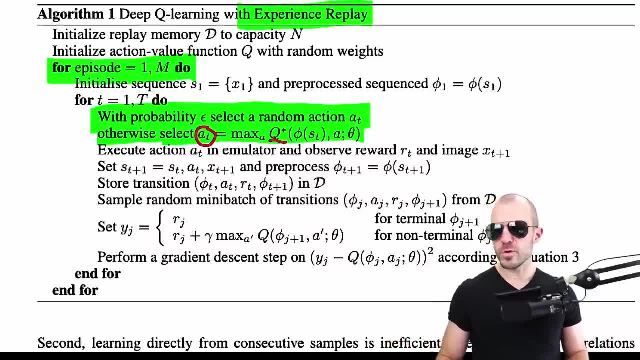 exploration because we, with high probability we will never reach the interesting states and or not enough, not often enough, and therefore we'd rather already start going along the good trajectories. as we learn the q function right and only with a small probability do something random, we explore a little bit. we don't get deceived by always going into what we think is the maximum. 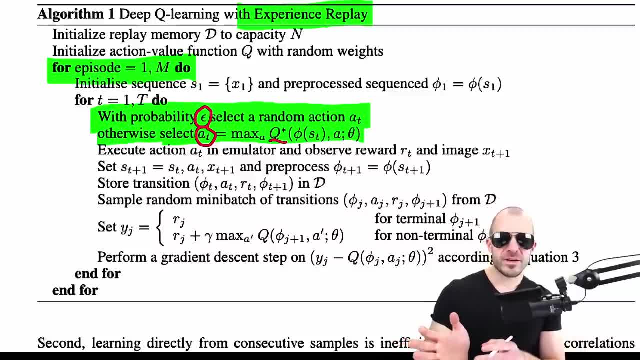 reward direction, because it could be that you know, right now i have to do a little bit of a sub-optimal move, but then there is much more reward and that's what the exploration is is supposed to do. it doesn't work in all environments and there have been 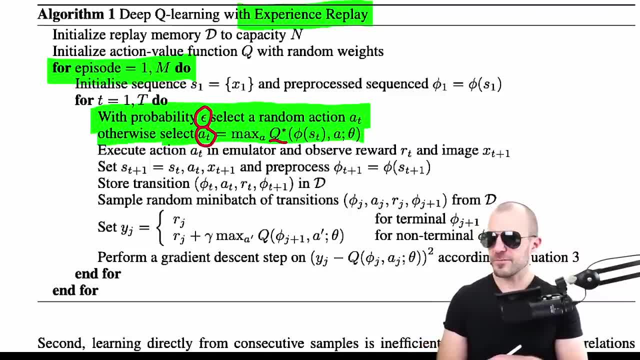 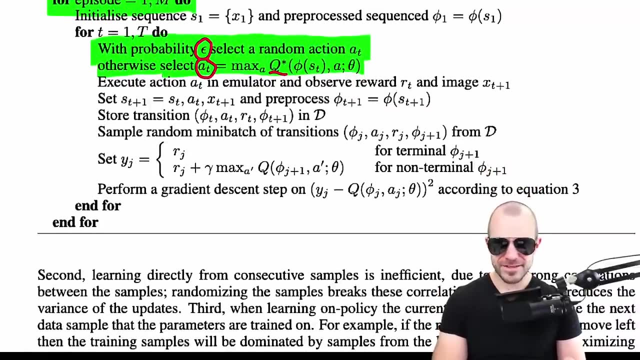 even books written about the deception of rewards and the deception of goals and so on, notably in even in the machine learning field, so don't don't recall what it's exactly called, but you'll find it. what they do, then, is they execute the action and they 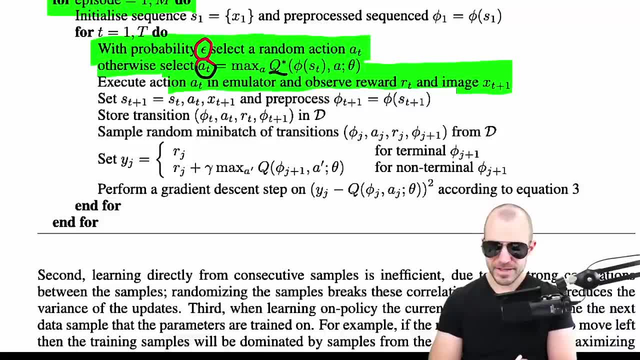 observe the reward and the next image. they set the next state to be okay. that's a step. they store the transition. eventually they'll sample a mini batch of transitions, so the transitions include the current embedding of the state, the action, the reward and the next. 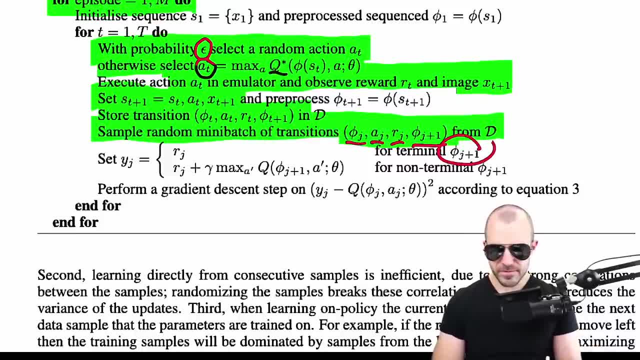 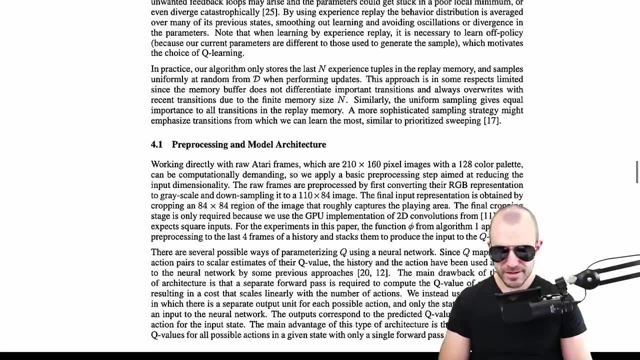 embedding of the state. If it's a terminal, they just set the target to the reward. If it's a non-terminal, they set the target to that Bellman recursion and then they perform a gradient step on the loss function. that we've seen before. And that's essentially it, And that's what gets you. 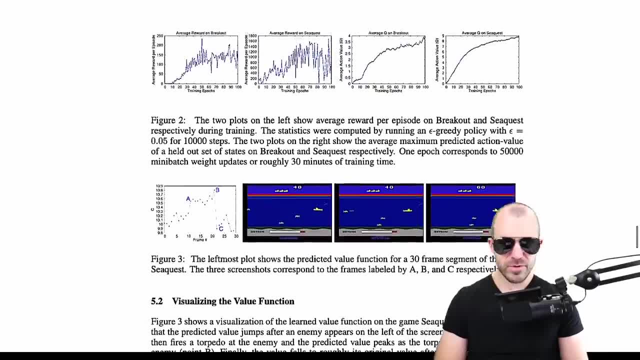 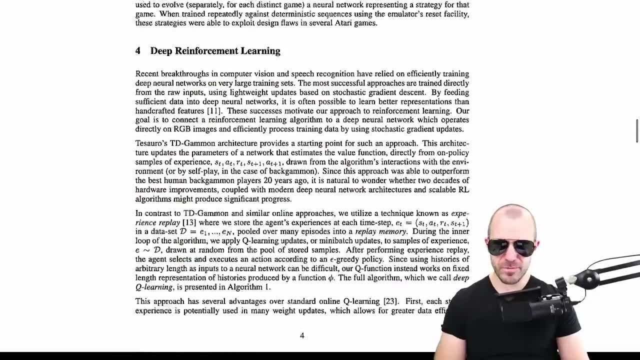 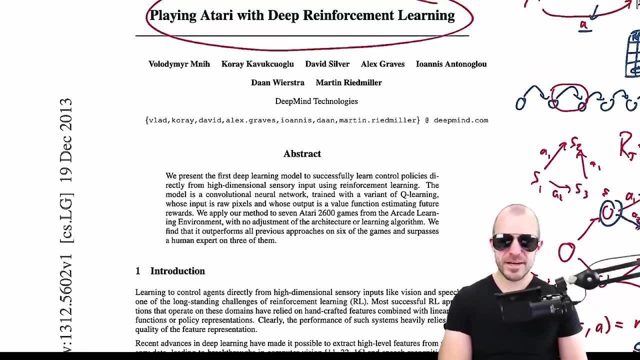 a giant super duper company that's getting acquired by Google, And I mean it takes a bit more than that, but this is really what put them on the map back then. So I hope this was a little bit of a dive into queue learning, into what it does, what it means. Again, we consider the queue. 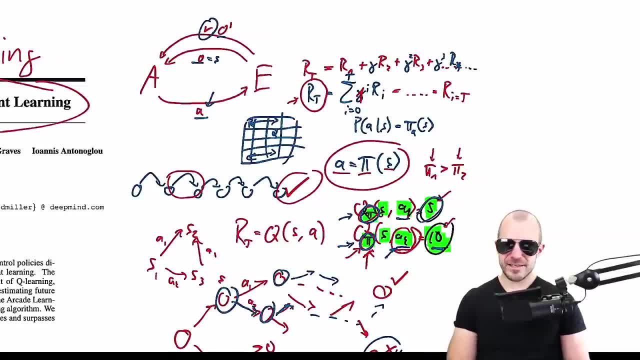 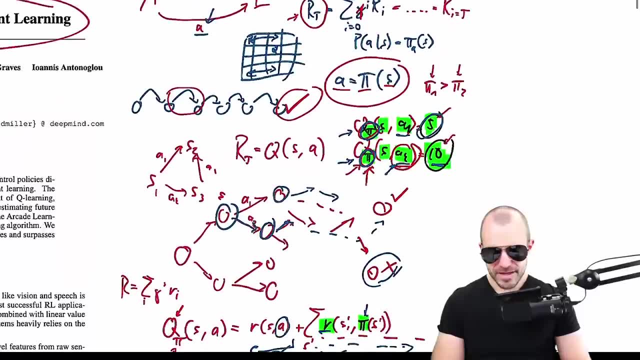 function, The queue function, is something that tells us if you did an action right now, if you did that in the state that you're currently in, what would the reward be? Not just now, but until the end of the game, If you follow, if you commit to follow a certain 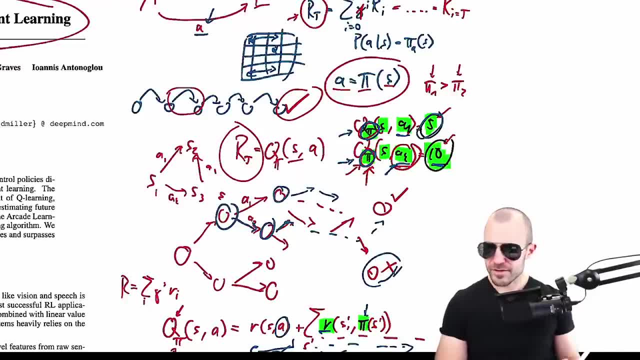 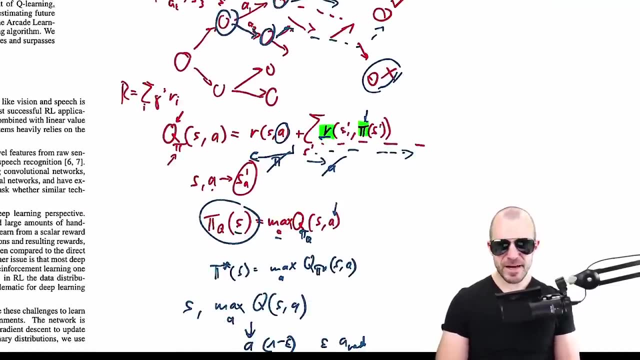 policy afterwards. and then we said: well, what if my policy is just? I'll always ask the queue function what I should do. And that led us to the realization that, hey, yeah, that's possible. In fact, it gives us a nice recurrence relation that essentially says: 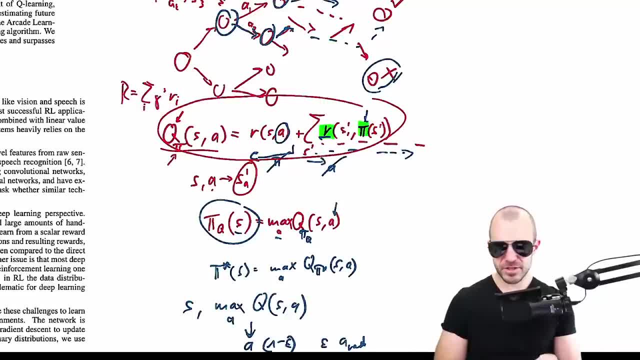 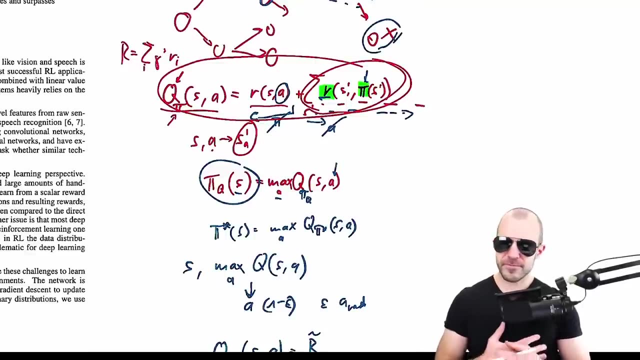 the queue function now is simply a combination of the reward that you'll get next step and the queue function of next step. That again led us to a method of saying, well, okay, that's cool, What if I don't know the queue function? Well then, I can just use the queue function to say, well, 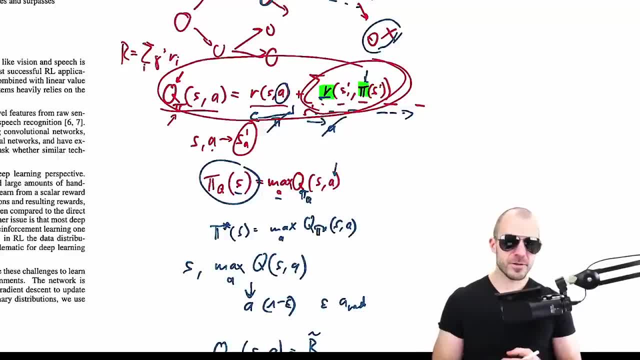 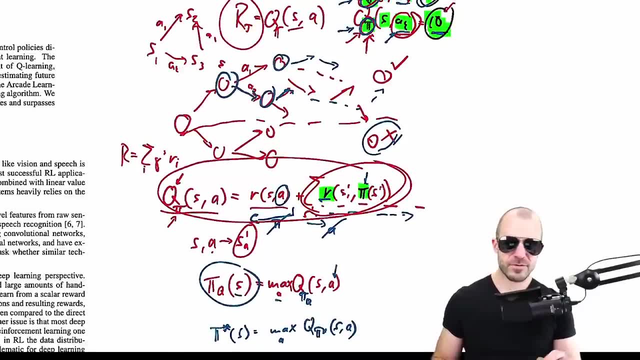 this recurrence relation to learn it, and learn it meaning I can break down the whole problem of what if the reward is like forever, and there are many steps and which is which, like which piece of reward is responsible for which action here, and so on this whole credit. 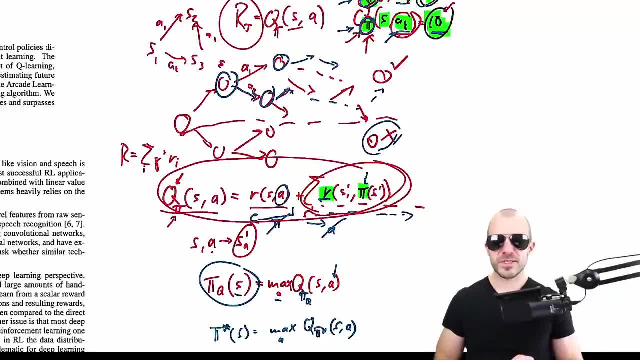 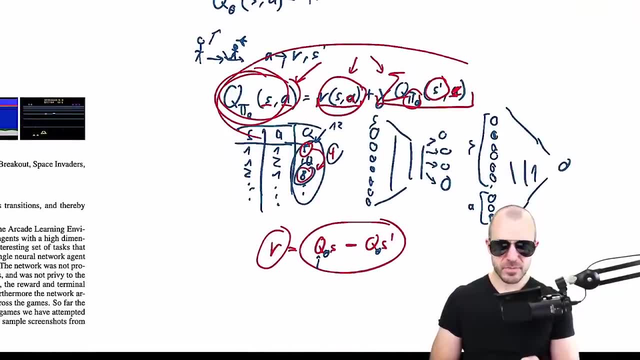 assignment problem. I can break it down into just learning from single steps, because I'm always saying, well, whatever else happens, the recurrence relation must be true For a single step. So the reward I get for a single step must be the difference between what 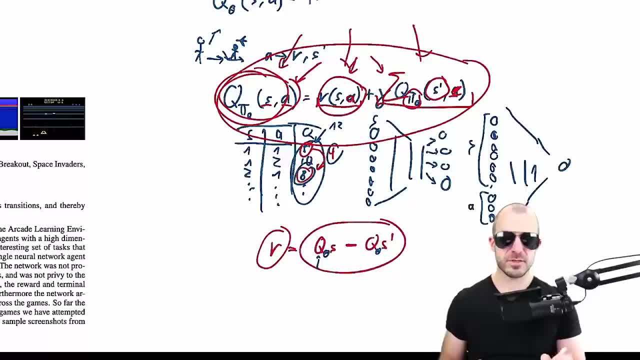 the queue function told me last step and what the queue function is going to tell me next step And that I can use to learn the queue function, at least the queue function of the optimal policy. And we discussed a little bit that initially queue learning was done really with 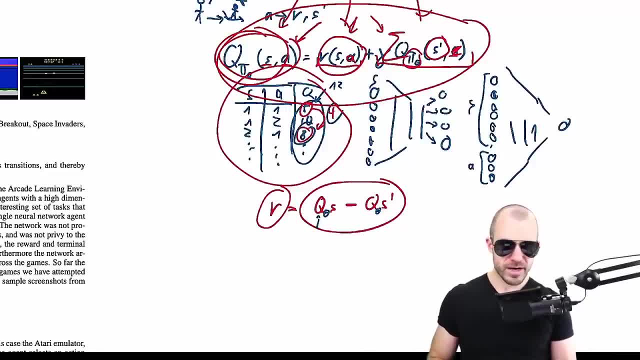 tabular queue values. But more and more as we move into modern ages, it can be done with neural networks, where you encode the state internal neural network and you ask the neural network you know for each of the actions. what would the output be? this could be done by having one head. 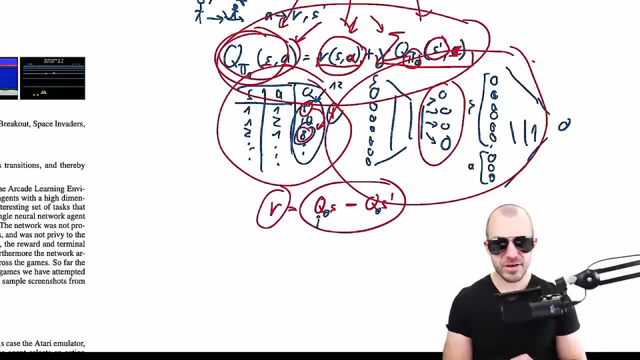 that just has an output for each available action, or by also encoding the action and then have one output And also encoding the action is going to allow us to go to a lot more complex actions, even continuous actions and so on, But we will not go over.